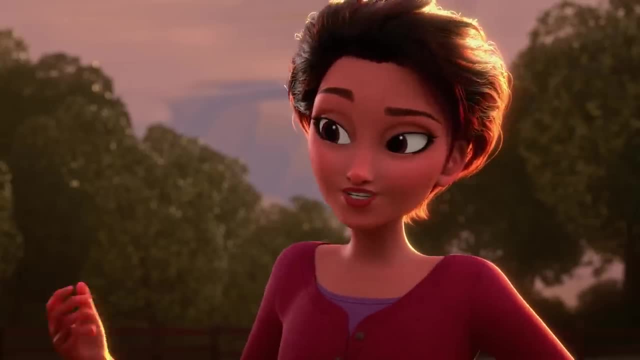 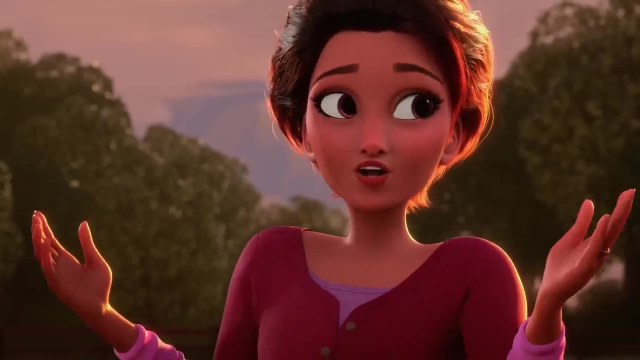 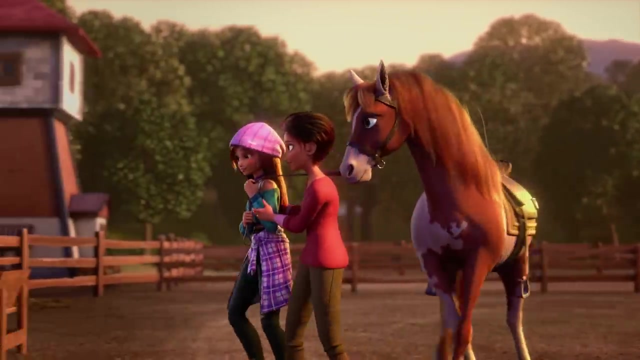 really. last week you rode in a thunderstorm to catch a chicken that got out. the week before you played tag with a bull fair point. why can't you ever do some non-dangerous, typical teenager stuff? you could make some friends go to the movies, have sleepovers. friends are overrated. 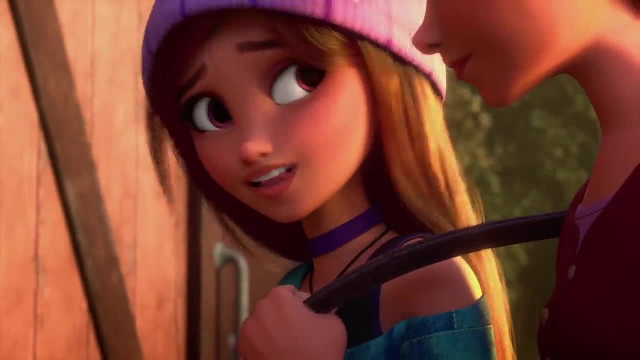 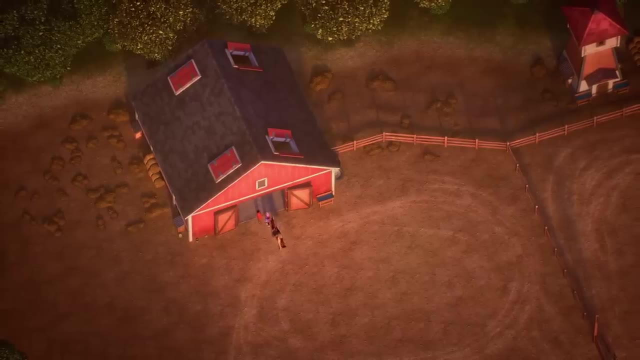 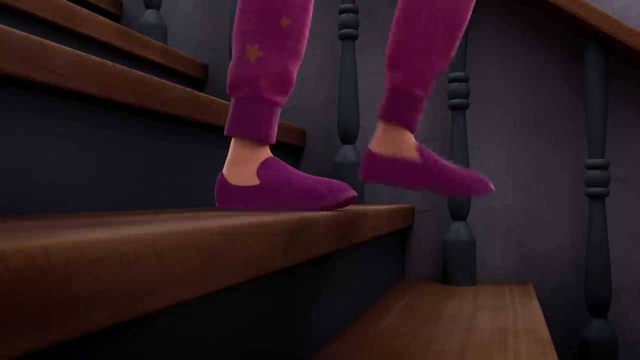 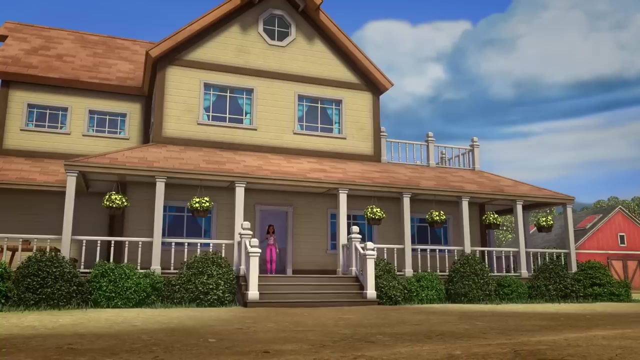 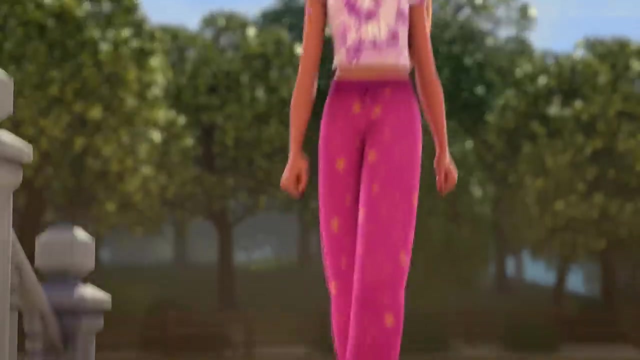 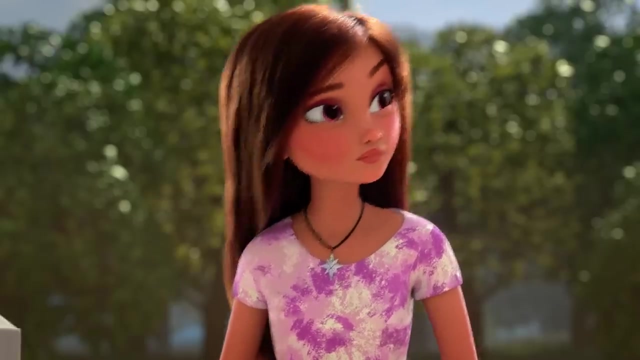 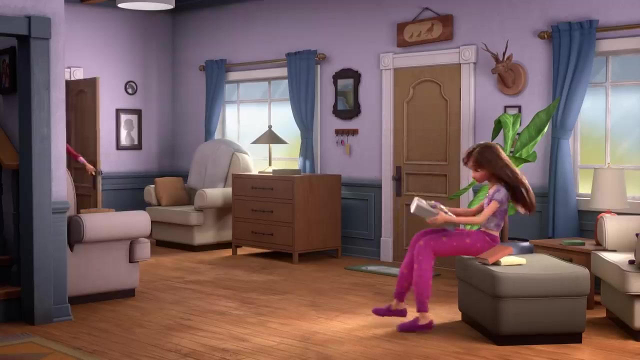 i'm more of a likably rebellious loner with a love of adventure that drives her mom nuts. you've got that right. oh and about you sneaking out grounded: yep, i figured morning, dad, i got it. hello, bubblegum, better hurry. if you want pancakes, your brother's a flapjack fiend. what's that i don't know. 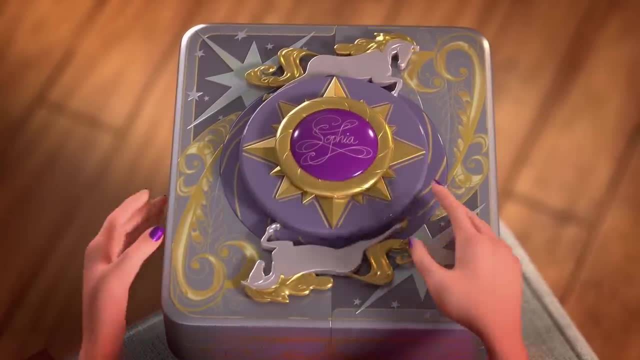 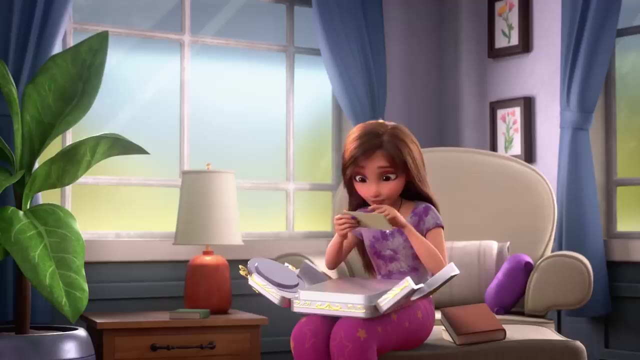 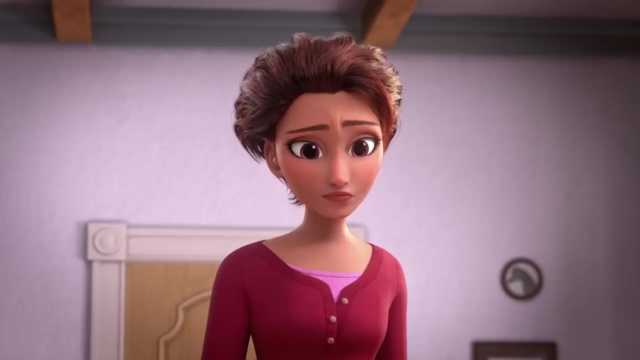 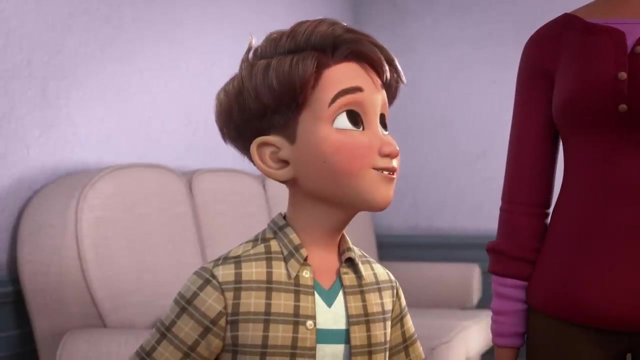 oh, we are. We are pleased to invite you to attend Nunzior Academy, the world's leading school for promising equestrian riders, A school where I get to ride all day. It looks amazing. Can I go? Can I have a room? 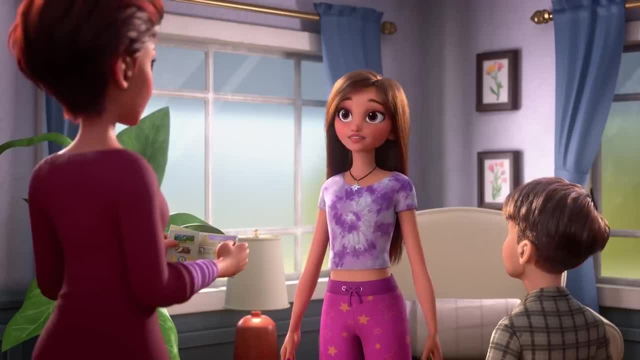 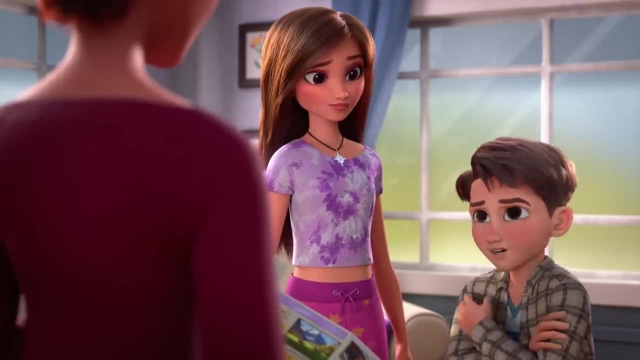 What about your school? here They don't let me bring a horse to class and it's not like anyone would miss me, But I would miss you, Marco, would miss you. The new bedroom would heal the pain. I'll go finish my pancakes. 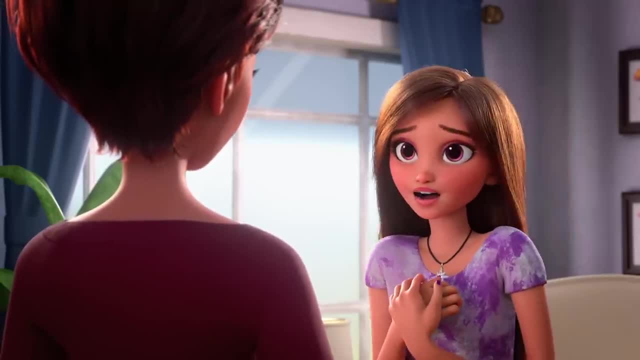 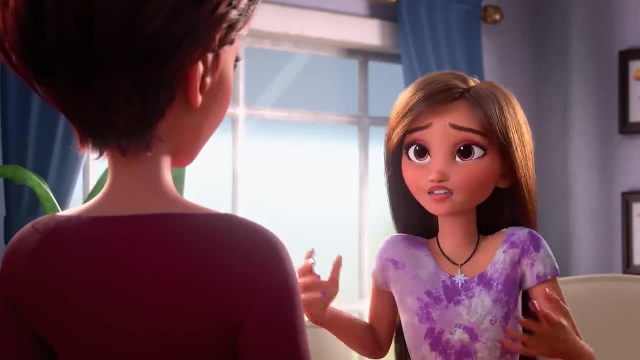 Mom, I know you worry about me, but I just have this feeling that I'm meant to do this. I'm sorry, but I don't think this is a good idea. What, Seriously, Mom? this is a riding academy. This is my dream. 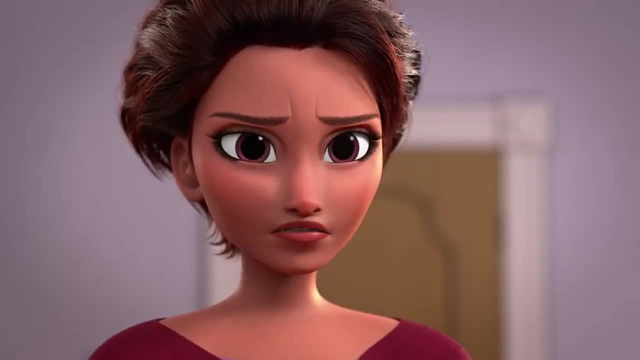 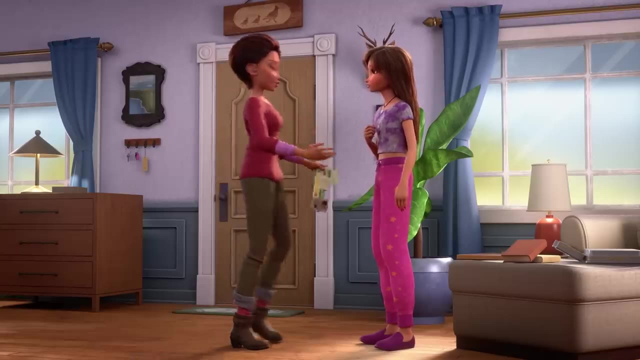 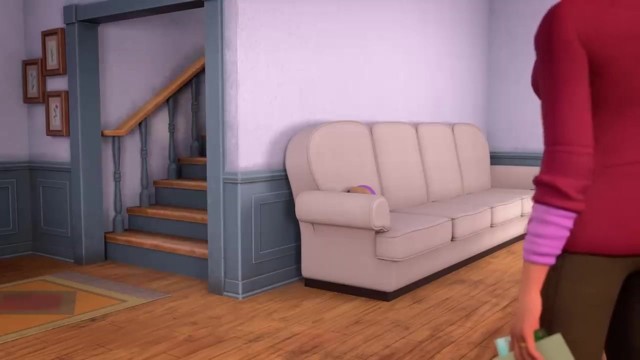 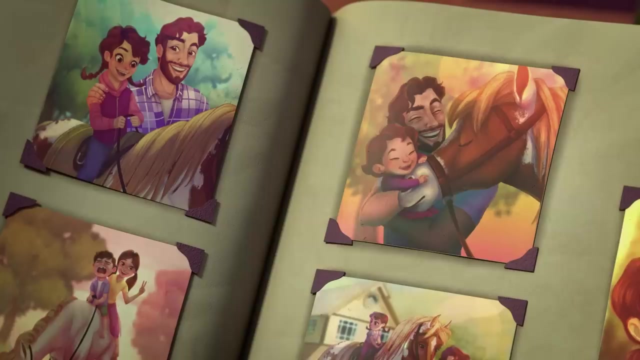 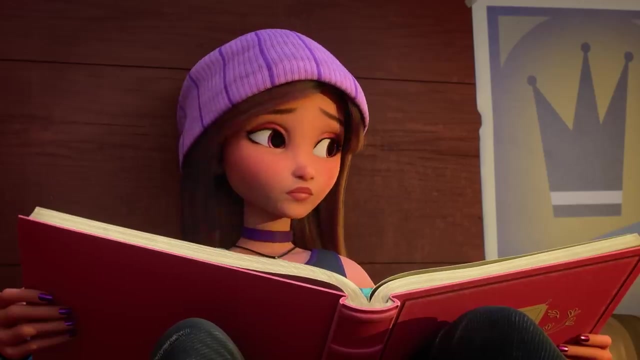 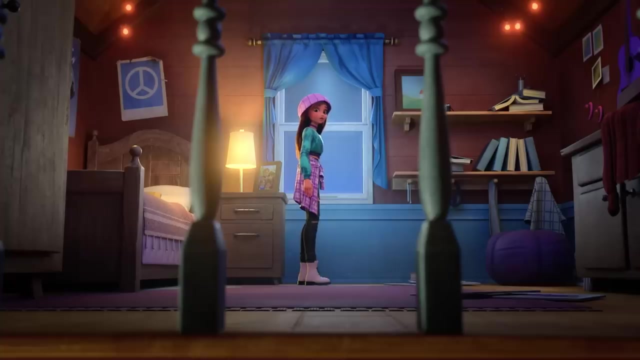 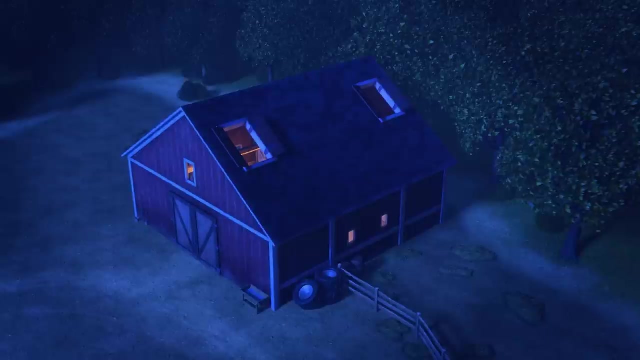 Dad would want me to go- If he were here he would- But he's not. Our family has lost enough. I don't want you leaving, Sophia. I don't want you leaving. I don't want you leaving. I hope I didn't get you in trouble yesterday. 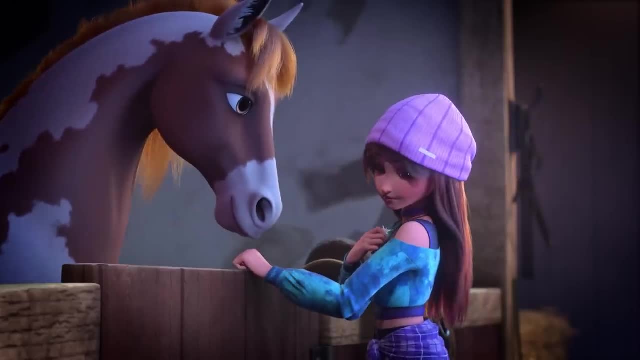 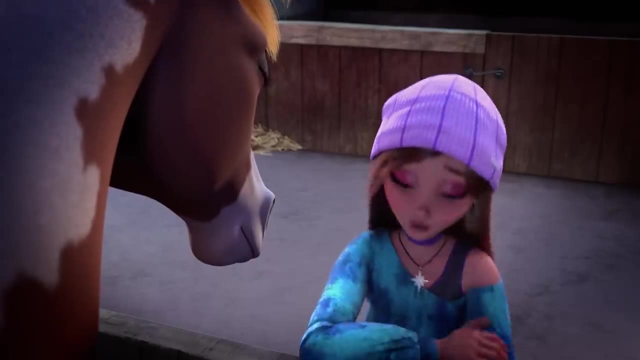 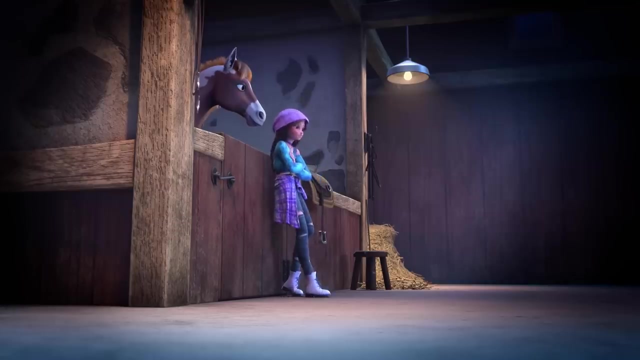 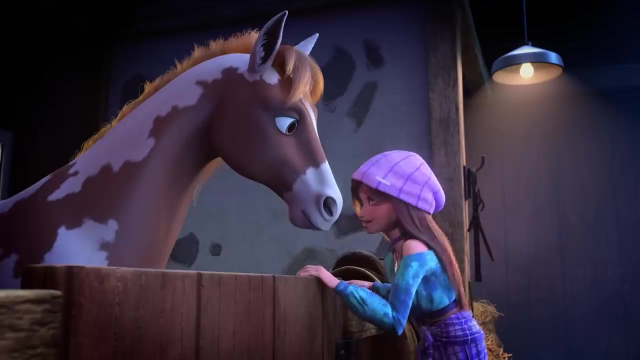 Mom doesn't get how much we need to run sometimes. Remember our rides with Dad. He always said it was destined for something extraordinary. I just wish I knew what it was. Do you ever feel like there has to be more out there, Like there's something inside of you? 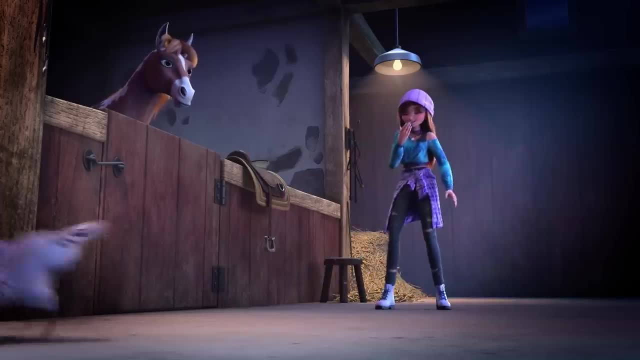 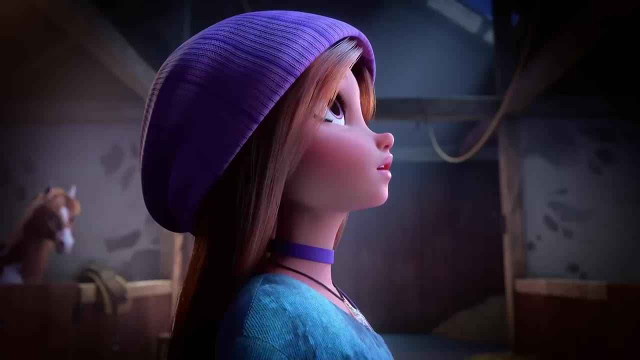 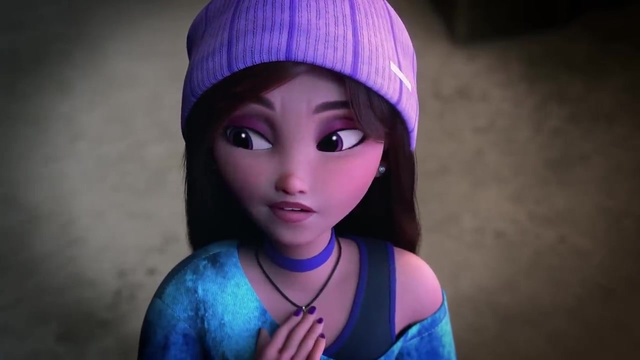 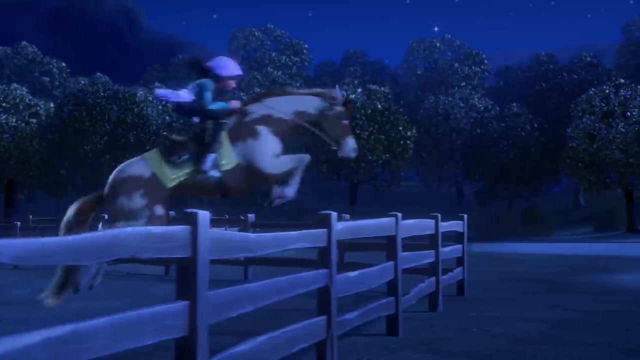 that's bursting to come out. Mmm, You do. huh, Ooh, Ooh, Oooooh. It just feels like the light burning brighter and brighter. I can't keep up. It feels like the light burning brighter and brighter. 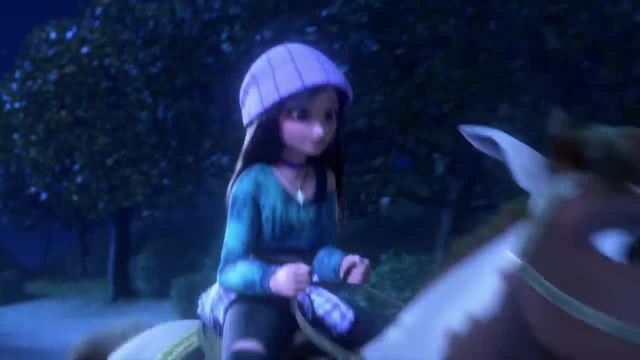 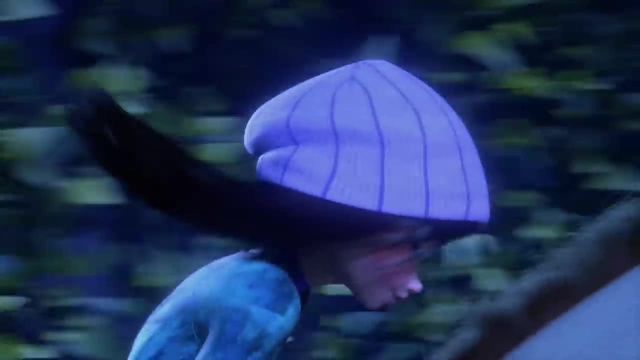 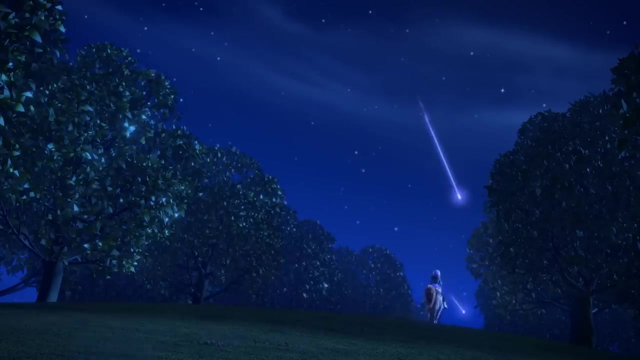 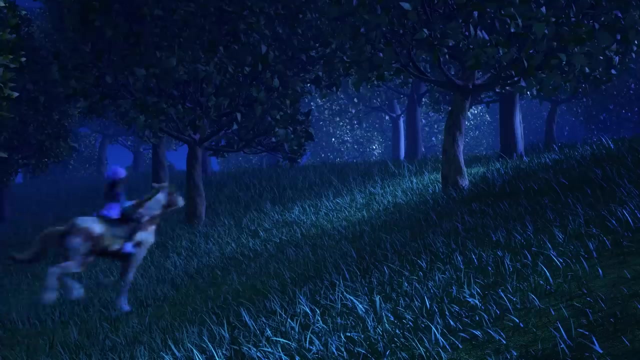 A feeling I just can't ignore, A pull to keep riding towards the horizon, To places I've not been before A world to explore. I've got to explore, You know, in those books where they're chasing adventure, That story is calling to me. If I know one thing: 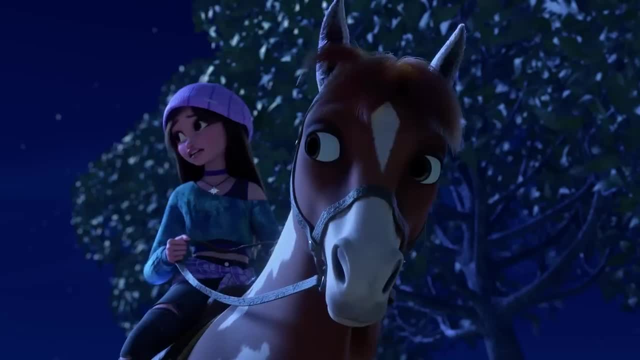 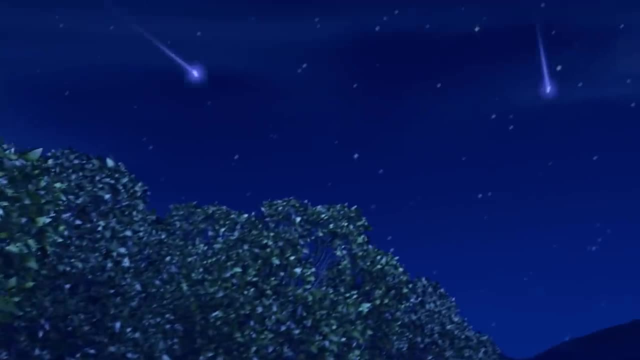 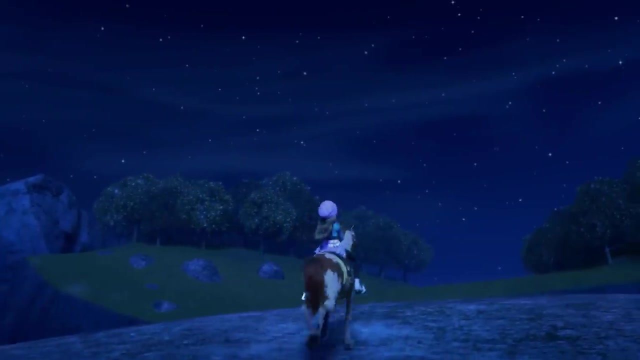 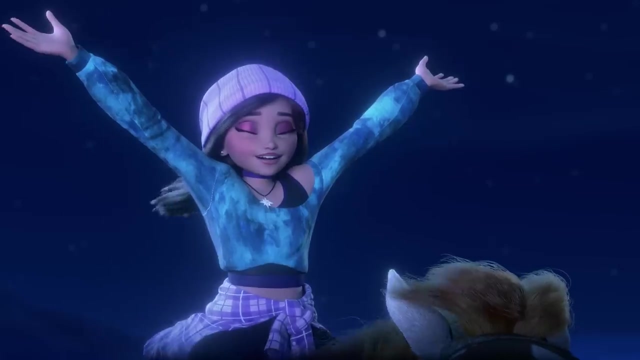 It's that staying in one place won't teach a girl anything. I need to explore. I'm ready for more. I have this dream of what could be A fire that's burning to be set free. There's a light inside of me, Fire. I feel the powerful winds of change. 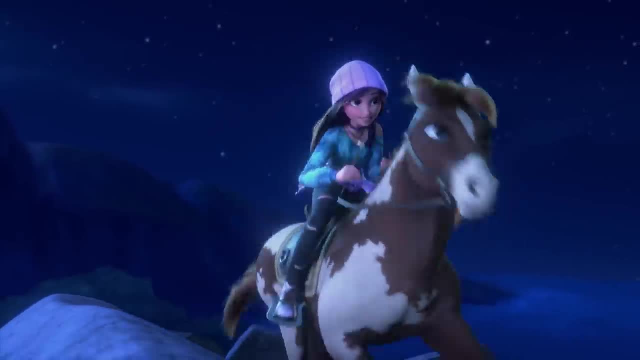 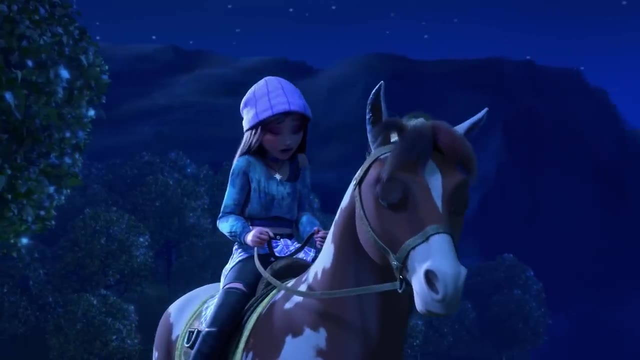 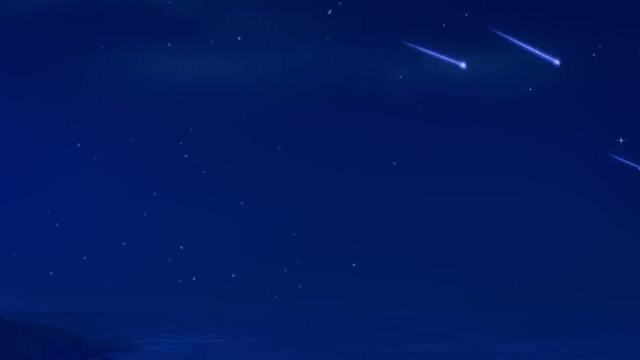 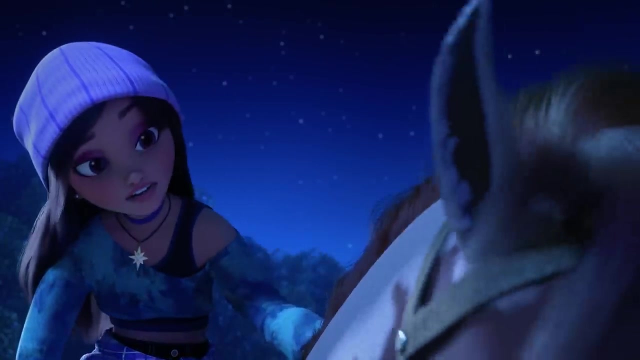 Guiding me somewhere. I know it sounds strange. Could this be fate Calling for me My destiny? And should I just follow this light inside of me? Fire, There's got to be a way. There's got to be a way. There's got to be more. 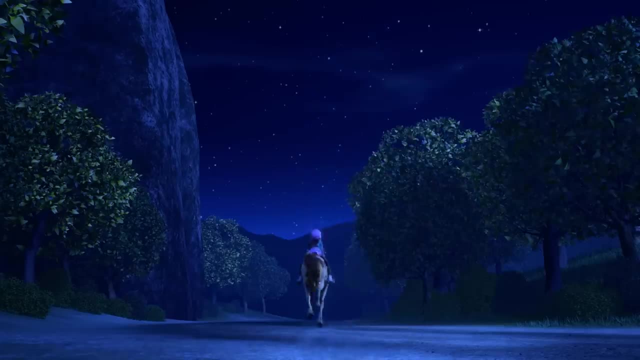 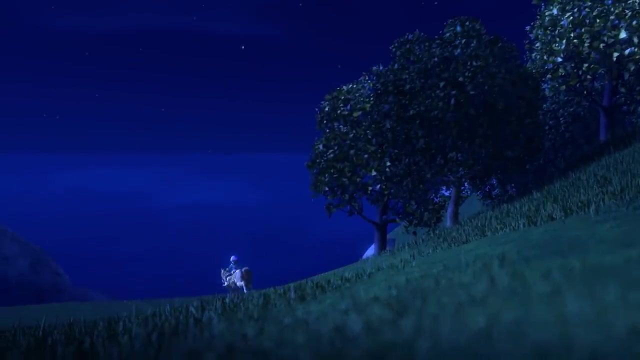 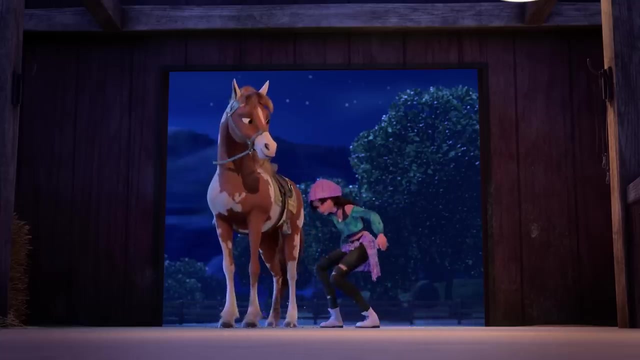 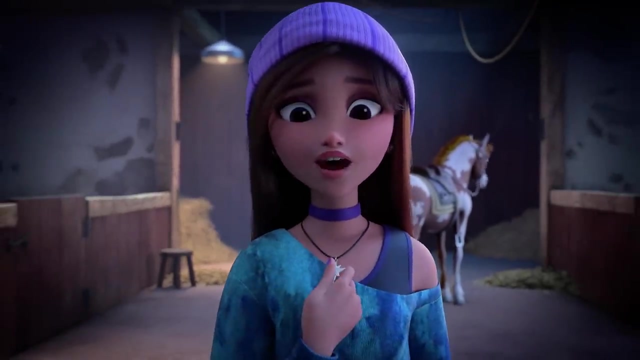 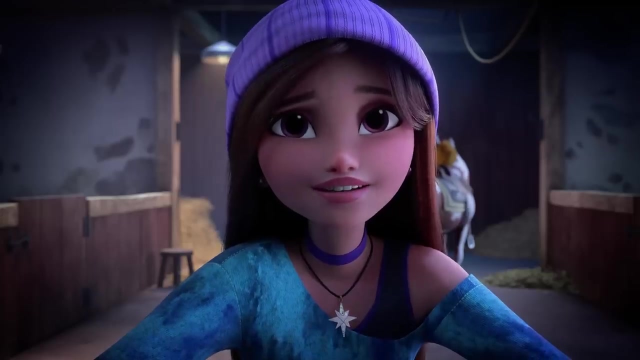 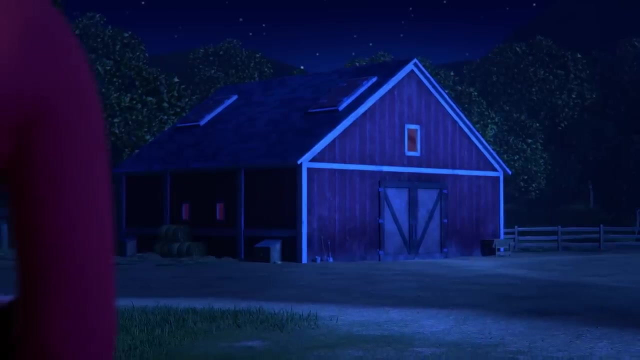 Got to be more. I have this dream of what could be A fire that's burning to be set free. There's a light inside of me. Who am I meant to be? The light burning inside of me? Is that what they call destiny Fire? Oh, 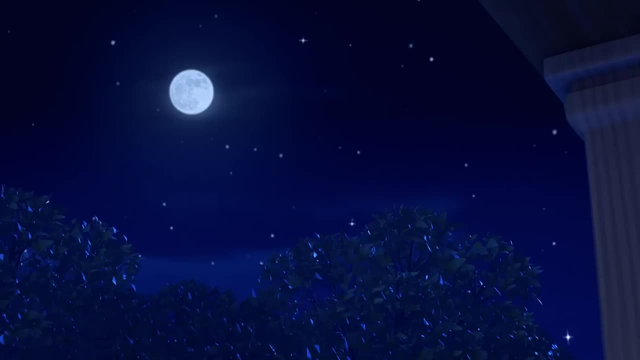 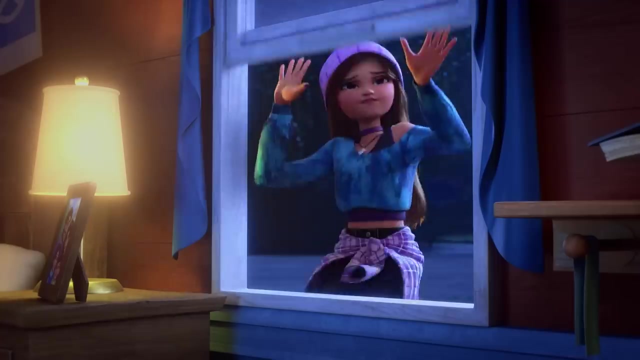 Uh, what is it? You know what? You feel: the fire inside of me. I feel the fire inside of me, Right in front of me. It's the fire inside of me. It's the fire inside of me. It's the fire inside of me, Oh. 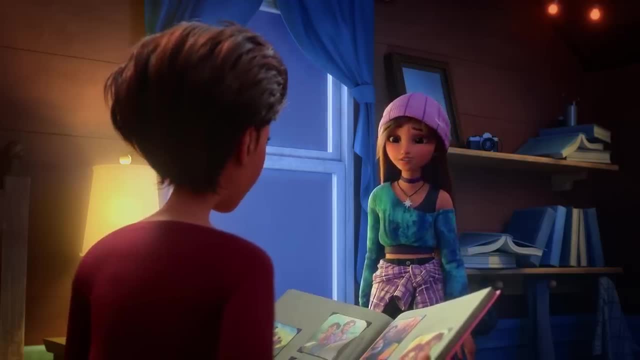 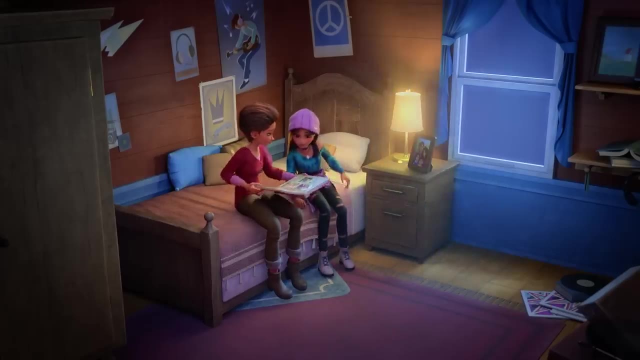 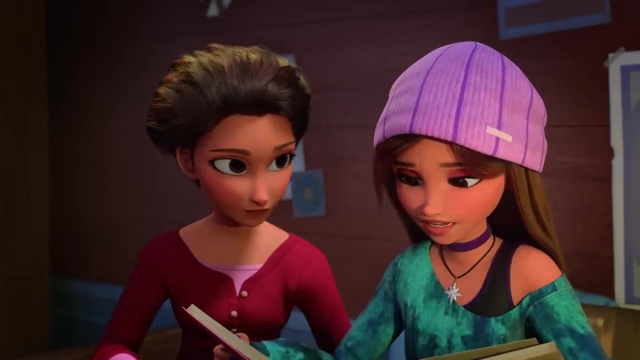 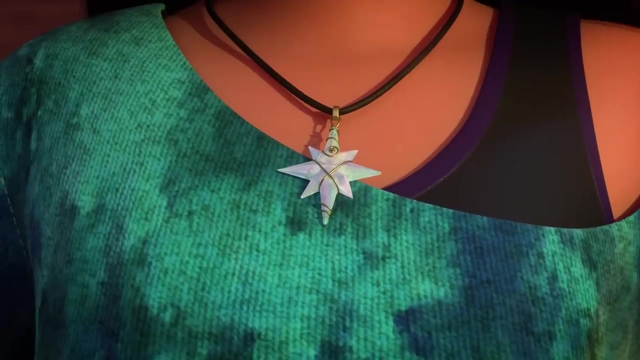 Is that what they call destiny? It's the fire inside of me. Uh hi Hi. I miss him too. I can't believe it's been five years. He'd love that you still wear the necklace he gave you. You were his shining star. 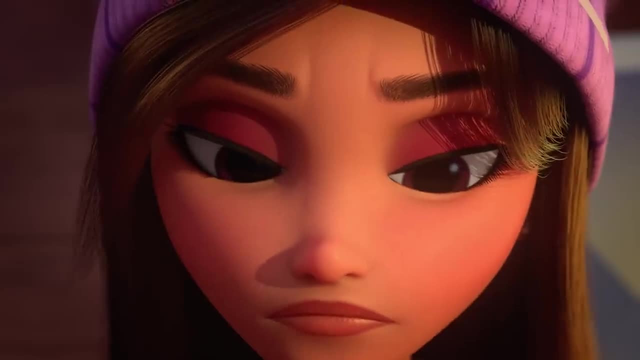 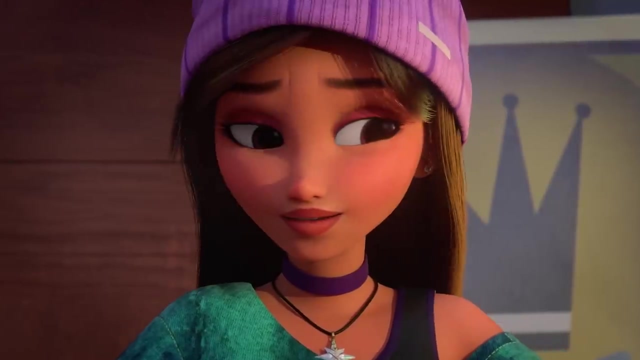 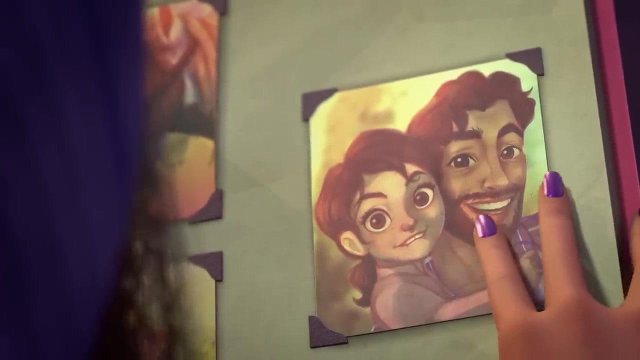 Sure, He'd also get a kick out of you wearing his old shirt, But it's definitely due for a wash. When we'd ride together, it felt like I could do anything, Like the whole world was there in my reach. Sometimes I just want to try and feel that again. 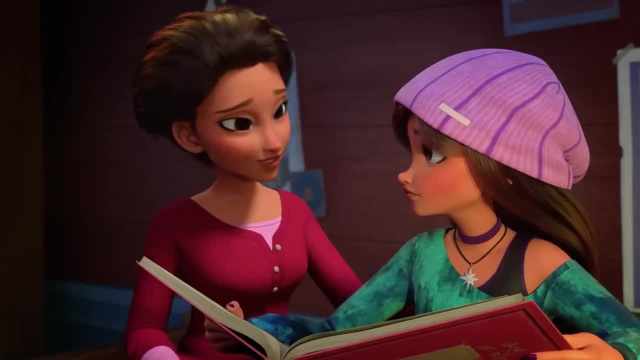 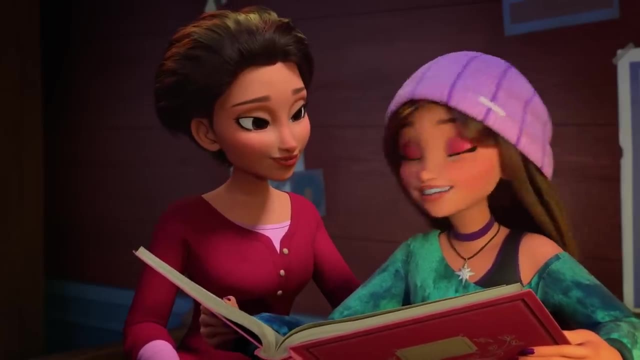 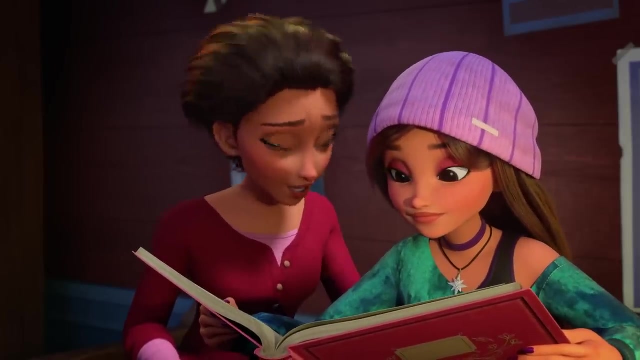 He loved you so much, Sophia. He had so many dreams for you. He would tell me you were destined for something extraordinary. You remind me so much of him. Do you know your dad also went to a riding academy? Really Wait. 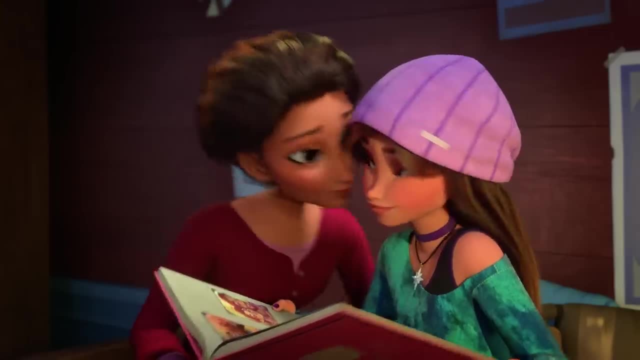 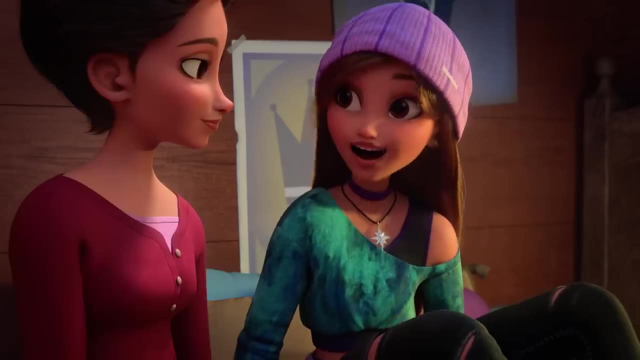 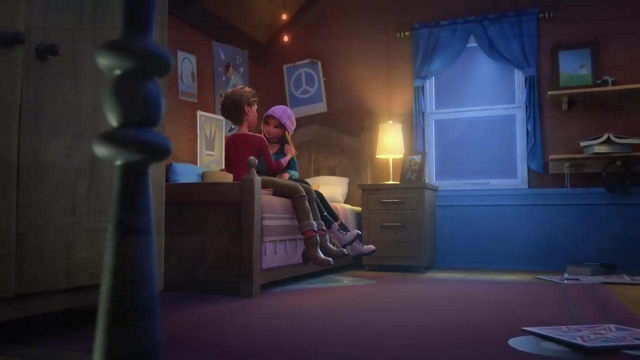 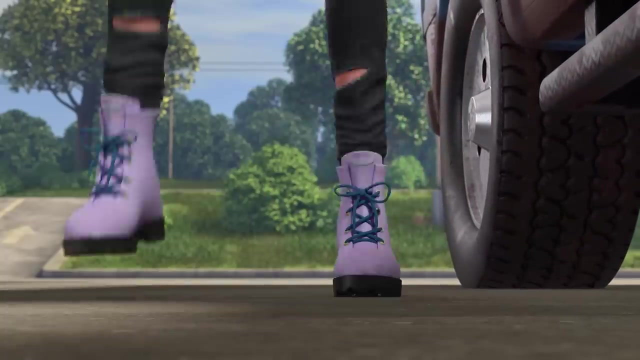 What do you mean? also, Better get some sleep. We've got a lot of packing to do tomorrow If you're going off to a new school. Thank you, thank you, thank you, We're here. There's my ride. 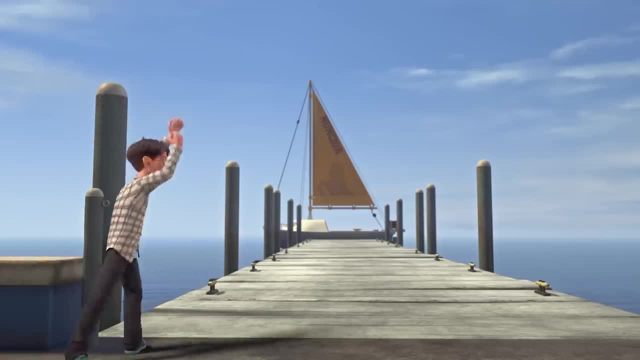 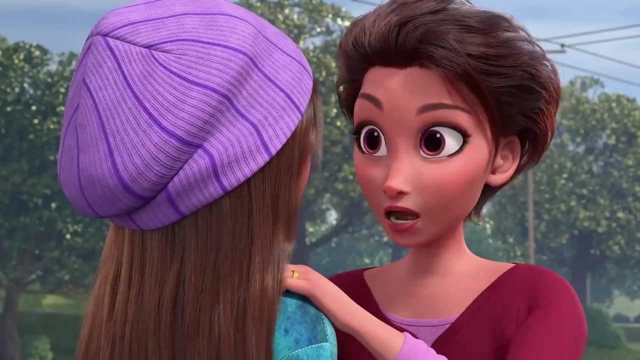 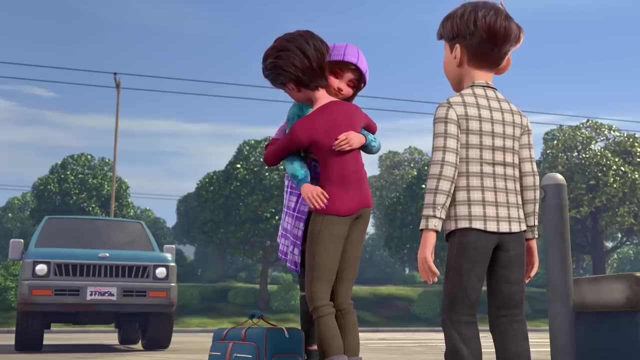 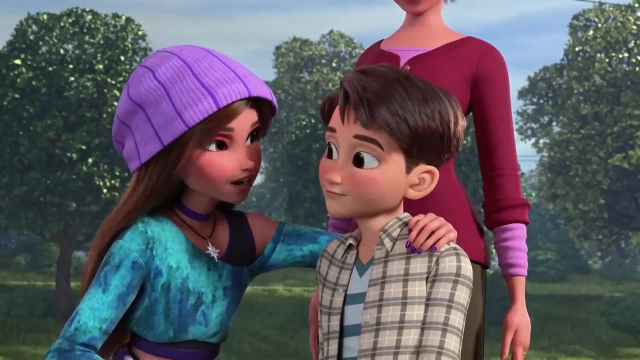 Whoa, Your school bus is a boat. Lucky Sophia, we're going to miss you, So call A lot. I promise, I promise, I promise. Now it's all on you to get into a little trouble while I'm gone. 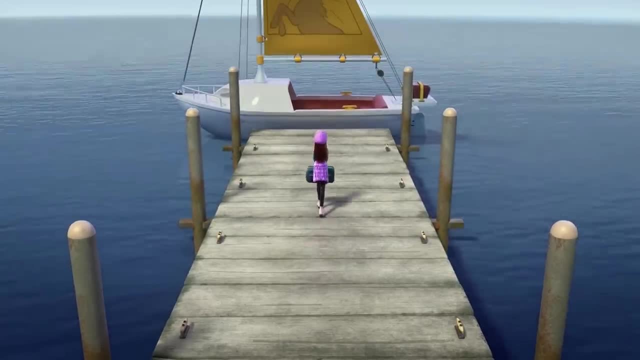 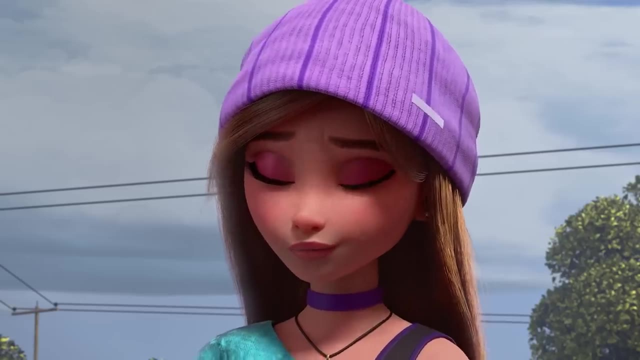 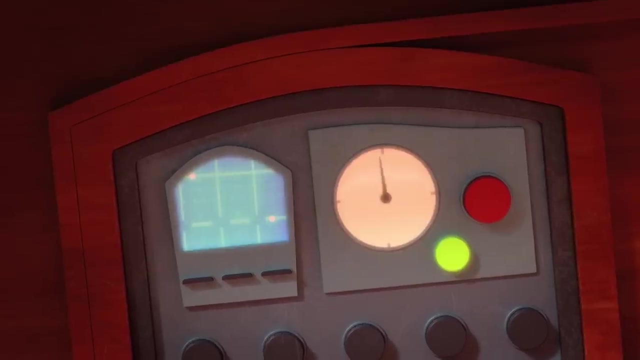 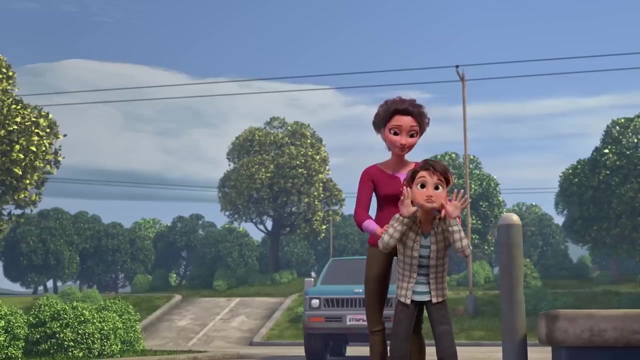 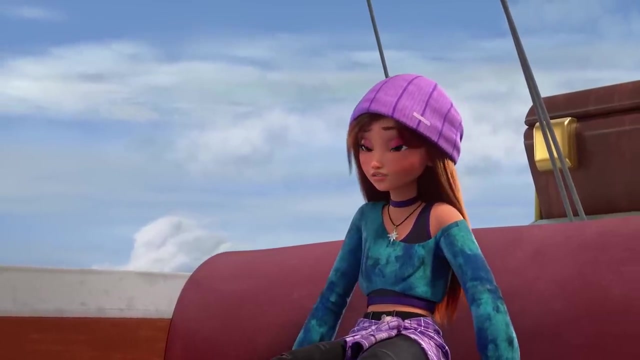 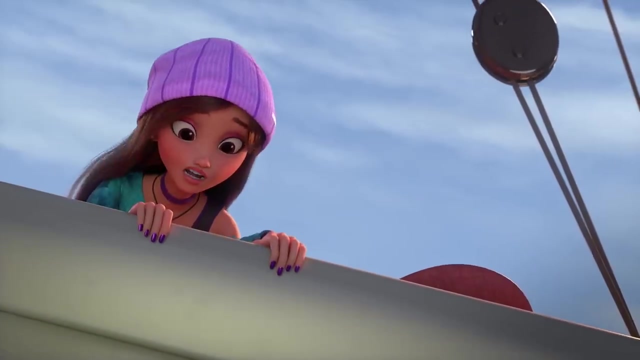 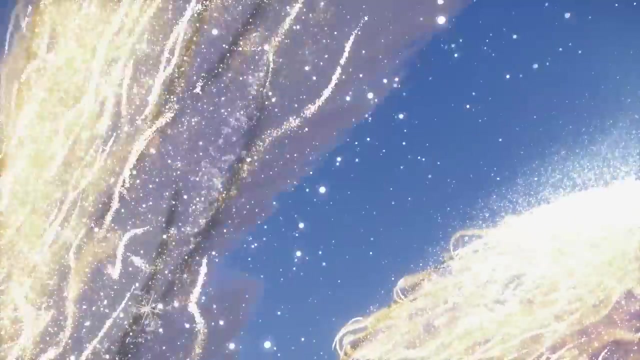 Bye. Thanks for the lift. I'm so fada- Huh, I've heard of driverless cars, but driverless boats. This academy is fancy. Huh, Huh, Ah, Whoa, Ah. What is happening? 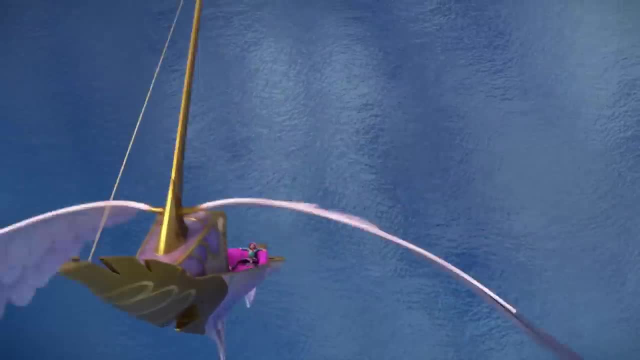 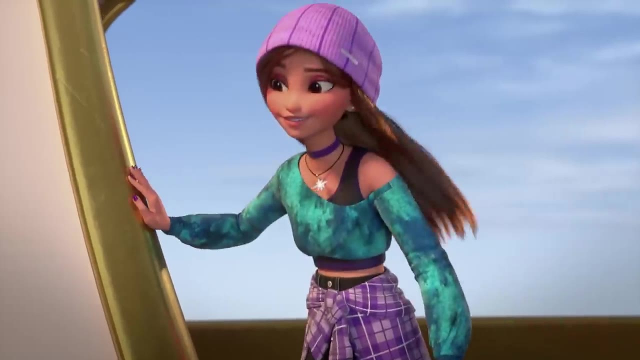 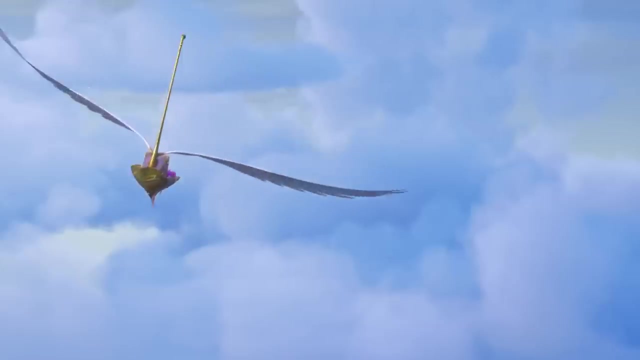 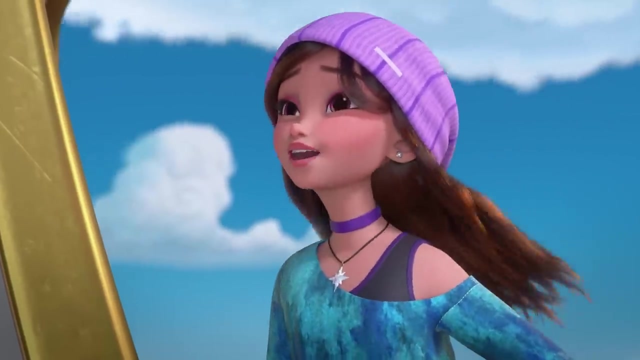 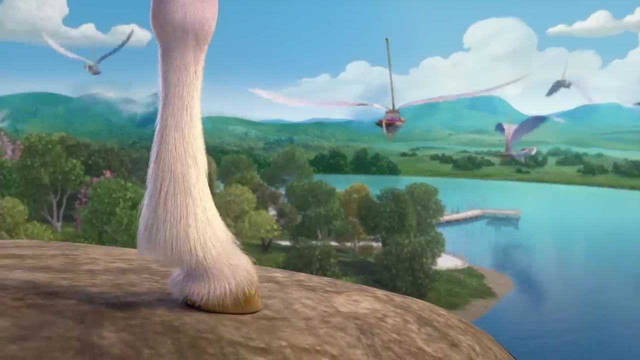 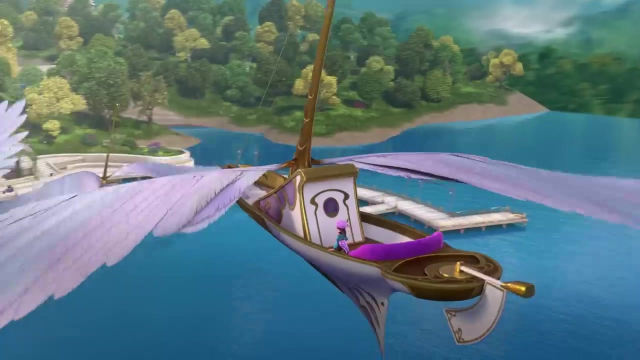 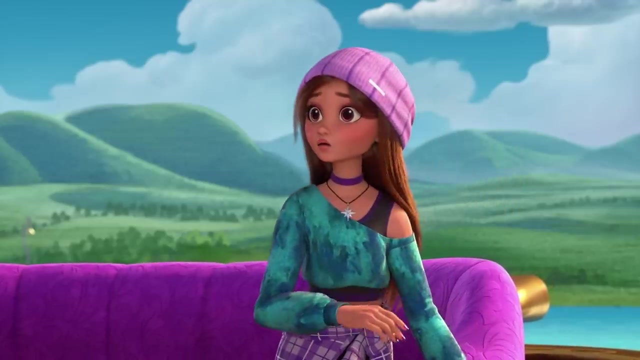 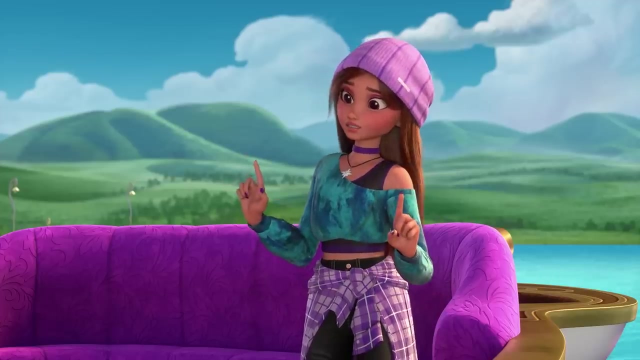 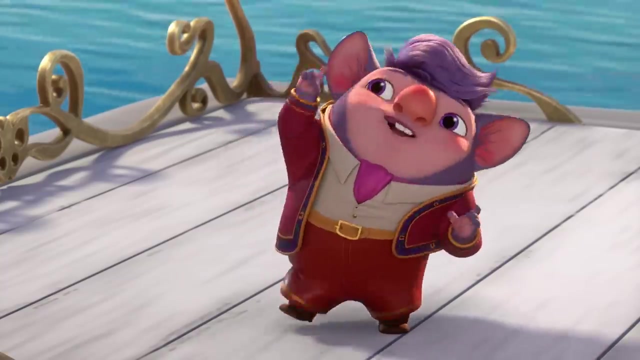 Ah, Ha-ha-ha, Woo-hoo. What kind of school is this? What? Oh? Okay, Sophia, you fell asleep and this is totally just a dream. Hello, Oh, it's no dream, But what a delightfully dreamy day. 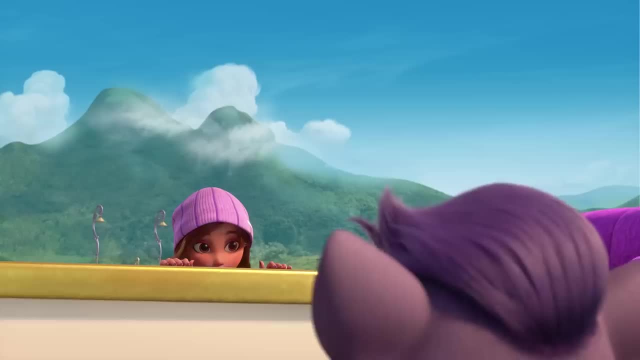 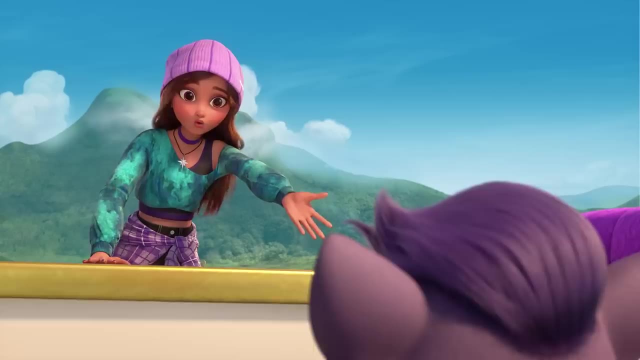 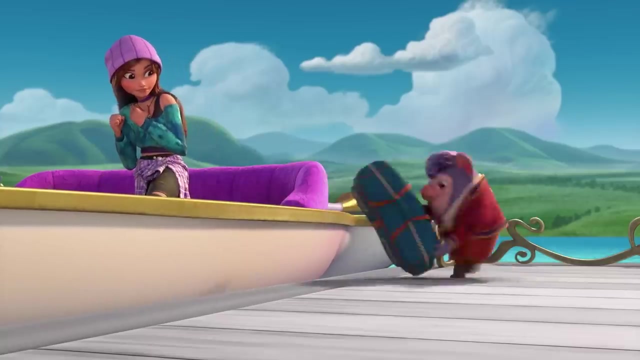 Sunshine with a crisp breeze. Did you have a pleasant trip? It was great, thank you, But uh, quick question: Where am I? who are you and when did they invent flying fairy-winged boats? Oh my, the talk is ticking. 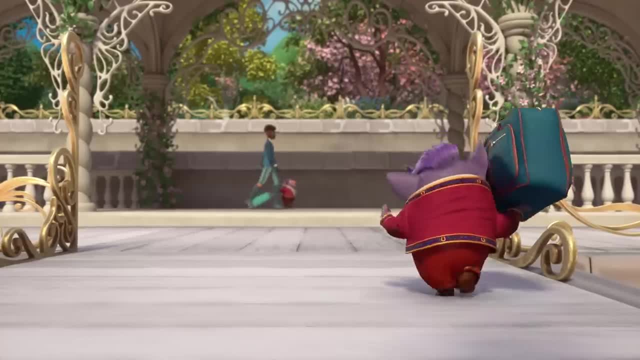 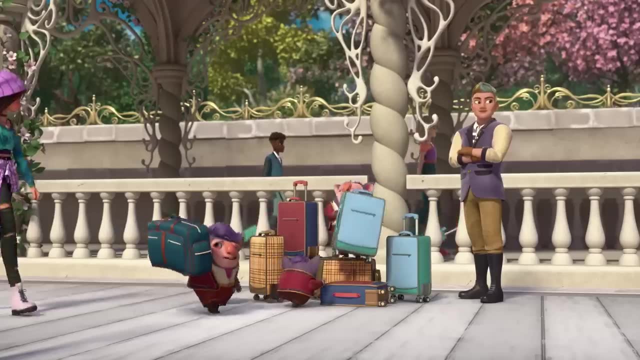 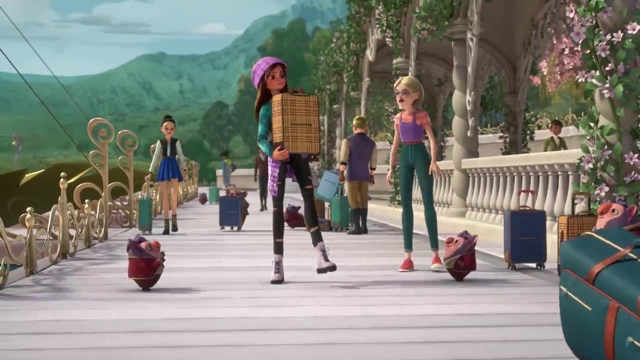 If you would please follow me. Uh, hey, I'm Furnicus welcome. Sorry, Huh, We Dwerpens have been assisting the day-to-day at the Academy for generations Dwerpens. what Sorry? Oh wait, wait, wait. 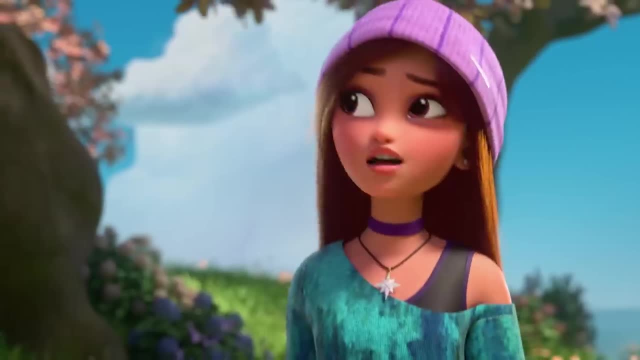 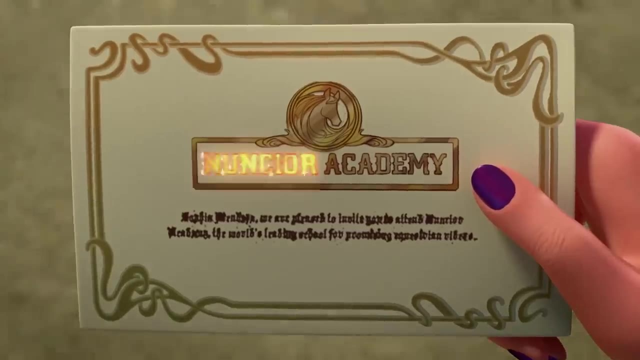 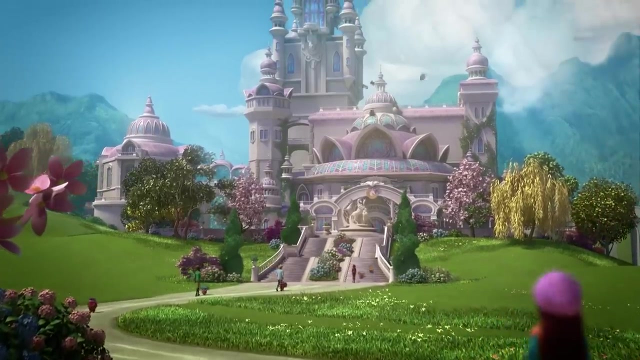 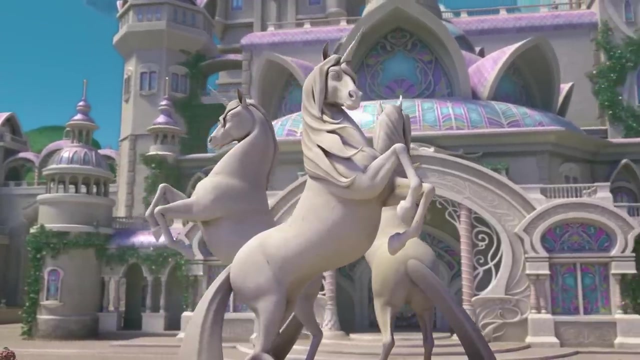 Look, Furnicus, my brain's about to explode. I thought I was going to a riding academy. You know, horses, a stable. I have the invitation right here. We are pleased to invite you to attend Unicorn Academy, Whoa. 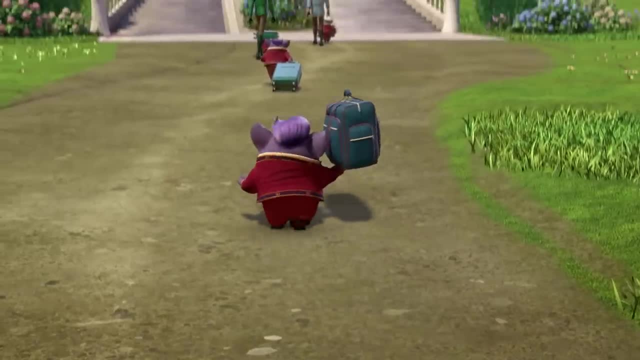 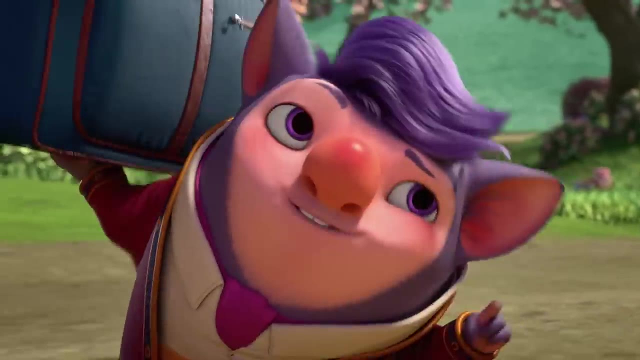 Come, come. orientation will begin in a few wiggles and a shake. Sorry, uh, unicorns. No, no way. Oh, I see You're one of those goofaloos who grew up believing that there's no such thing as magic. 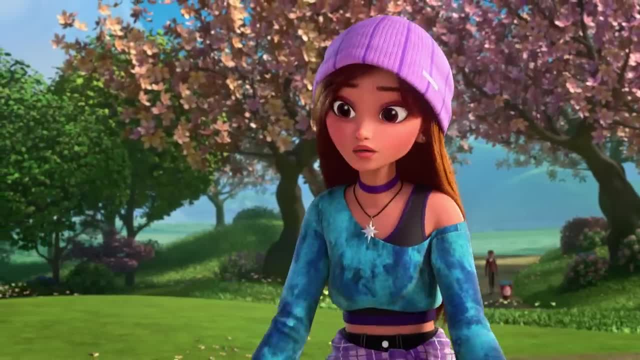 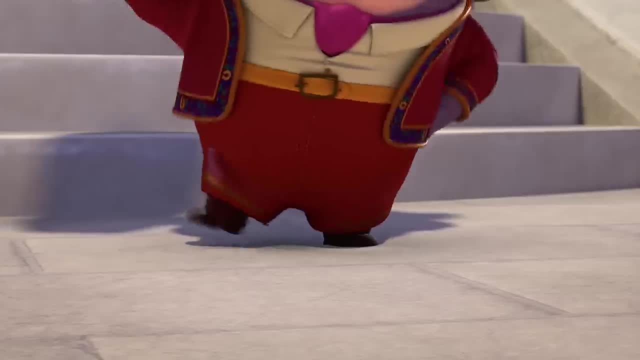 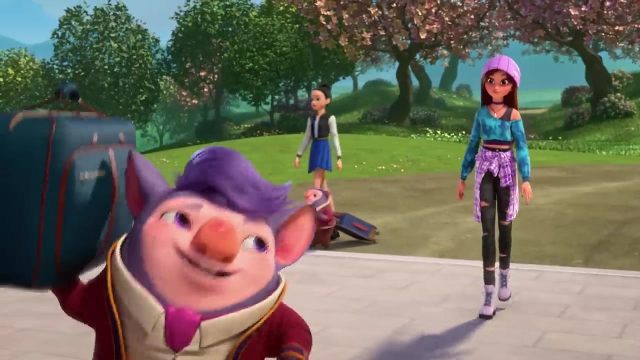 that unicorns aren't real Because they're not. Next, you'll be telling me that Dwerpins don't have two left feet. Wait, do they? Mom's a word about this place. But magic is real, as you or me, and Unicorn Island is the source of it all. 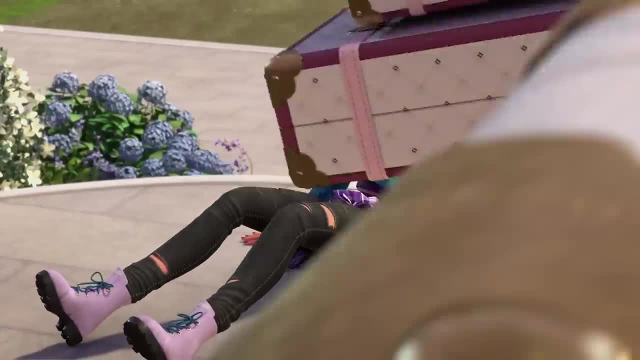 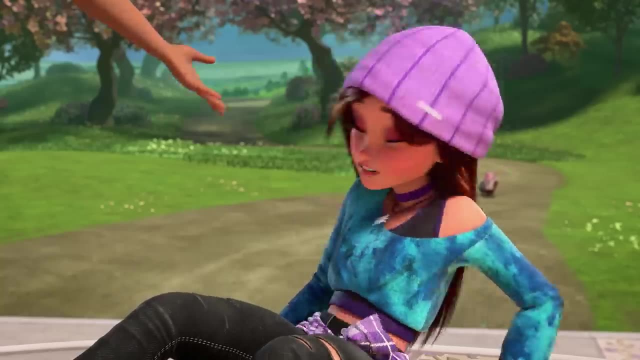 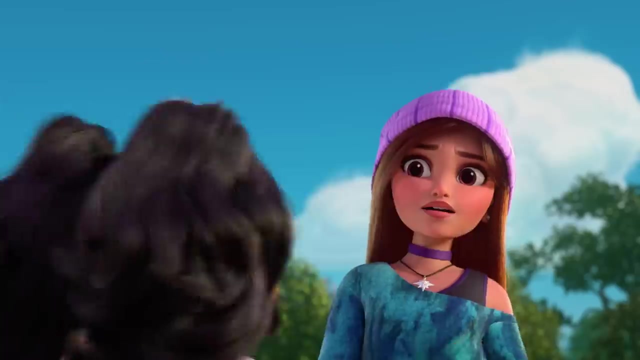 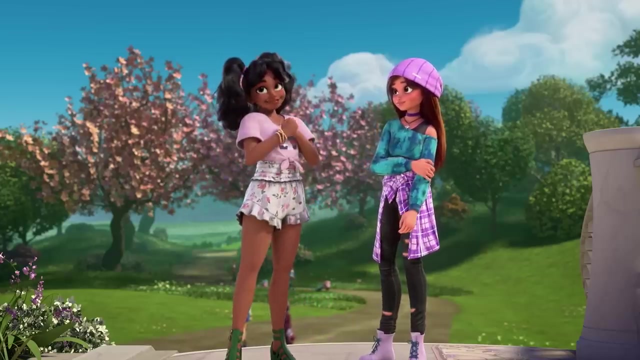 Excuse me, Ooh, I love your shirt. Purple is one of my 19 favorite colors. I'm Ava. It's so nice to meet you. Um, okay, I'm Sophia. Ooh, I have loved unicorns for literally forever. 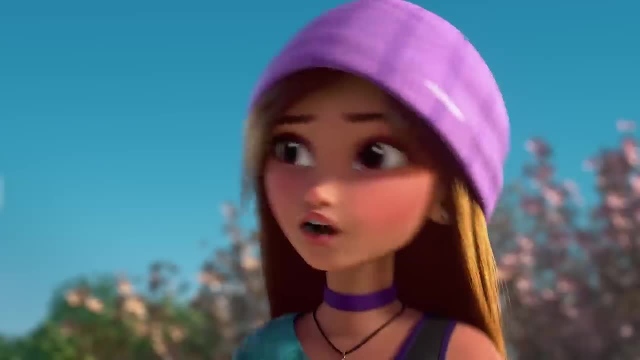 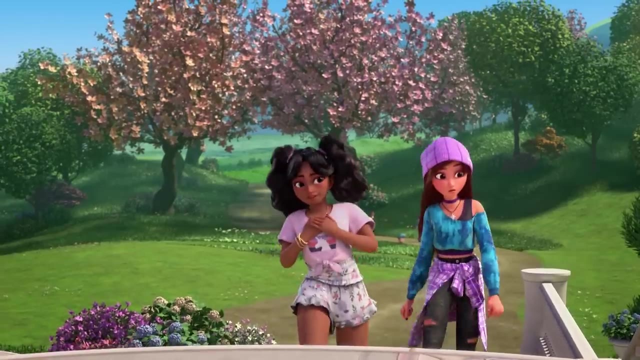 Can you believe we're actually here? Uh no, I don't believe any of this. Oh, You're not a legacy. My brothers went here and when I got my invitation they secretly told me everything. You must be totally confused and weirded out. 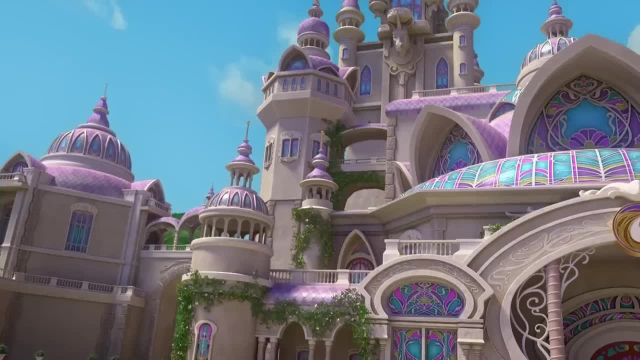 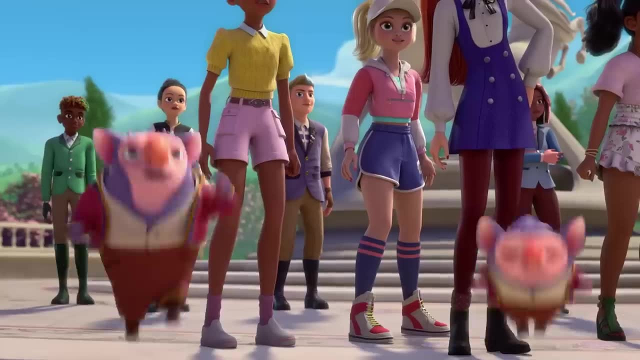 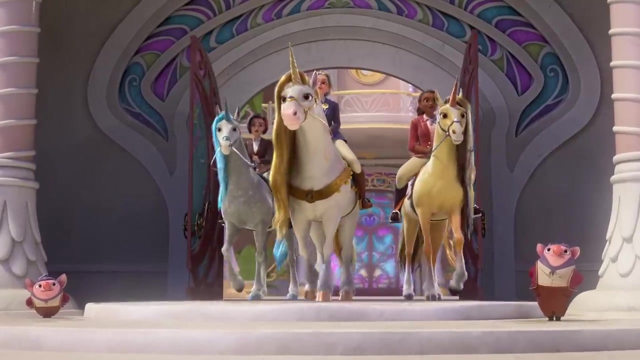 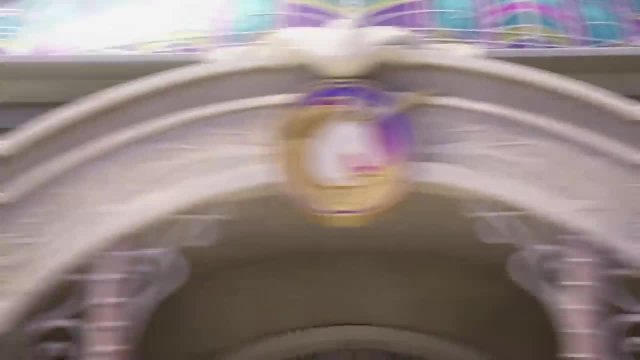 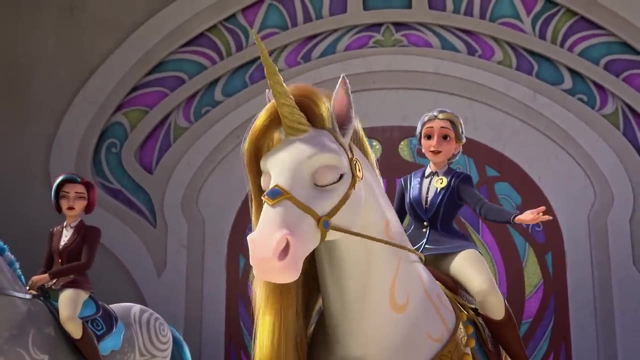 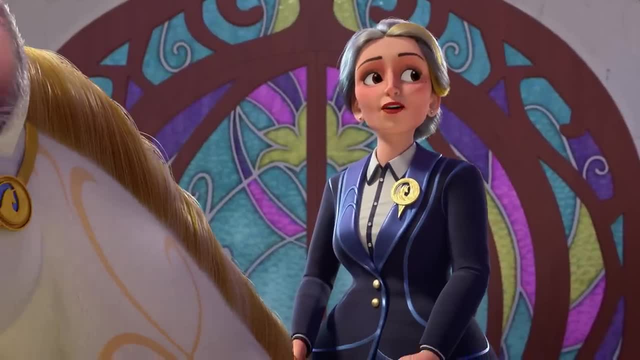 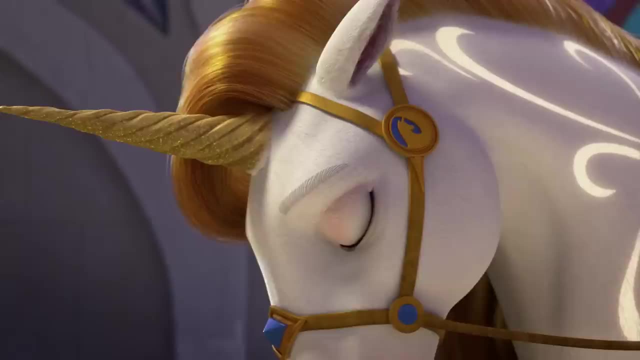 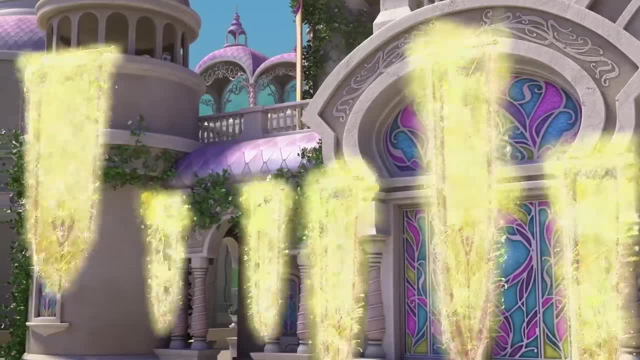 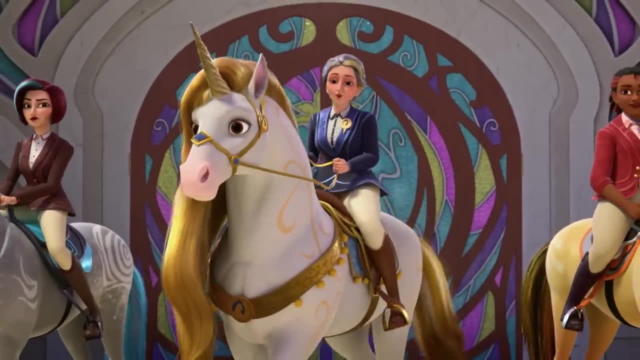 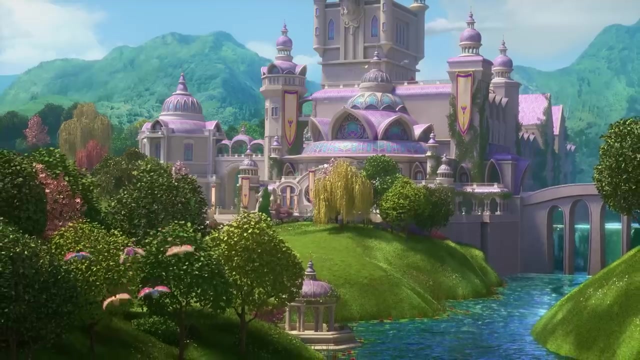 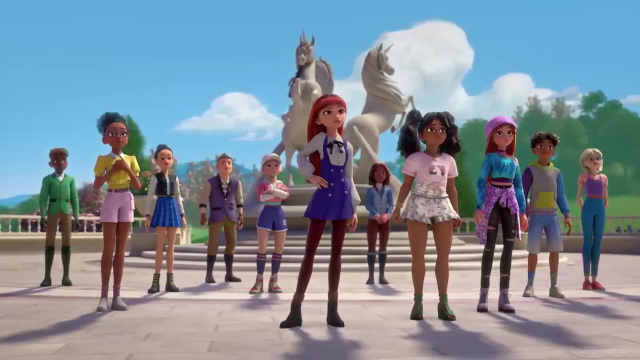 That's more like it. I'm Miss Primrose, head teacher at Unicorn Academy, And this is Unicorn Island. All the world's magic comes from here, And unicorns are its protectors, The only creatures mighty enough to keep the island safe from danger. 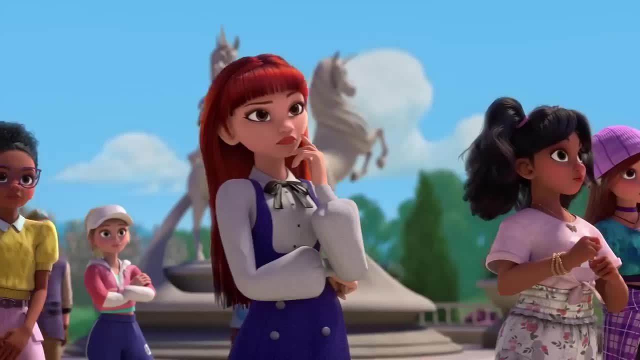 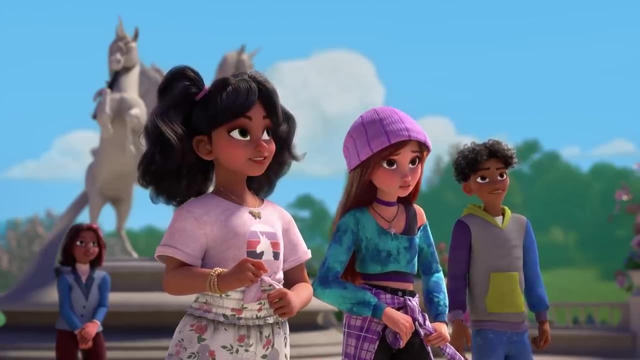 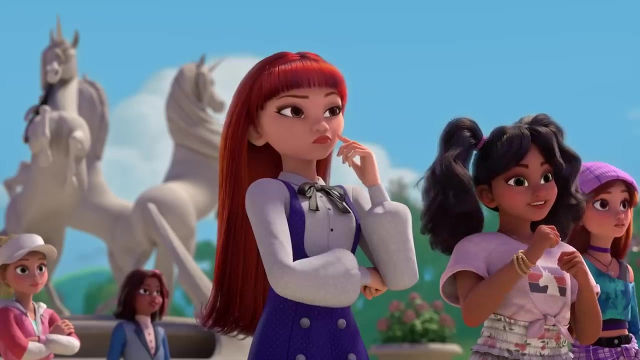 You have all been invited to join a long history of unicorn riders- Definitely not the kind of riding academy I expected. Some of you have been chosen for your extraordinary skills and talents. Others follow in the footsteps of a family member who was a unicorn rider before you. 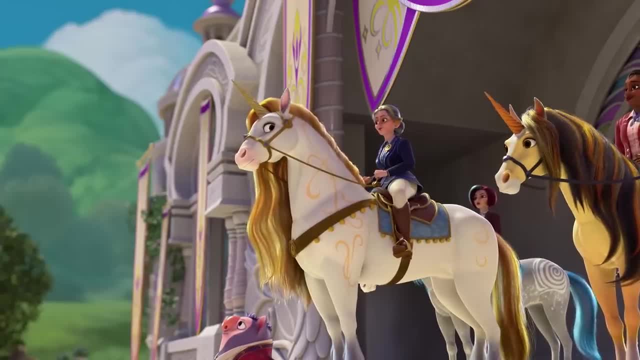 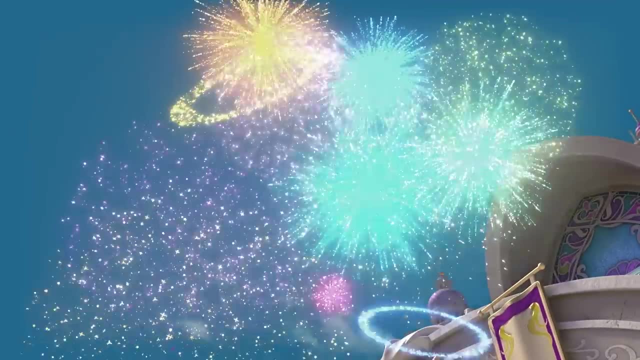 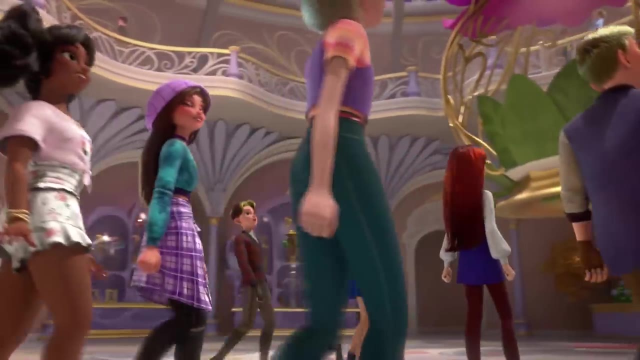 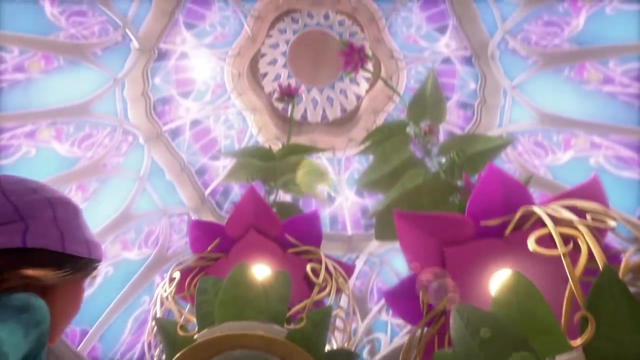 All of you have the potential to bond with a unicorn. Now get settled. Your journey begins tomorrow. Wow, Wow, Whoa, Hey, Come on, Can you believe it? Wow, This place is Incredible. New students gather for room assignments. 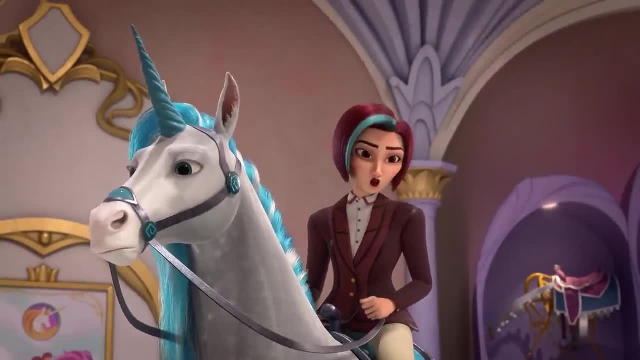 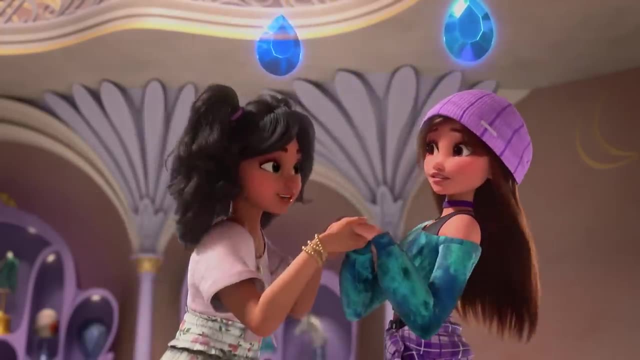 The fate fairies will select a gemstone that best suits you. Proceed to the chorus room. We're both in Sapphire Dorm. It's fate. I just know we're going to be besties. Boom, We're there. Hashtag: dream life. 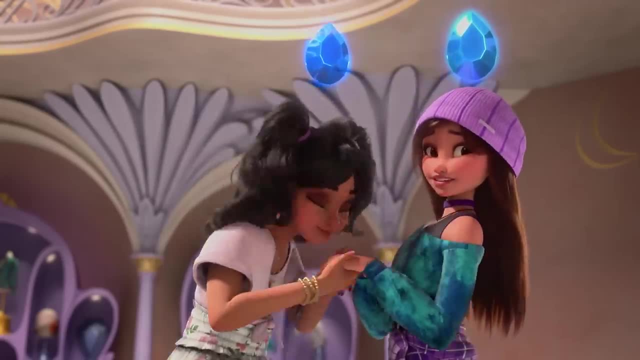 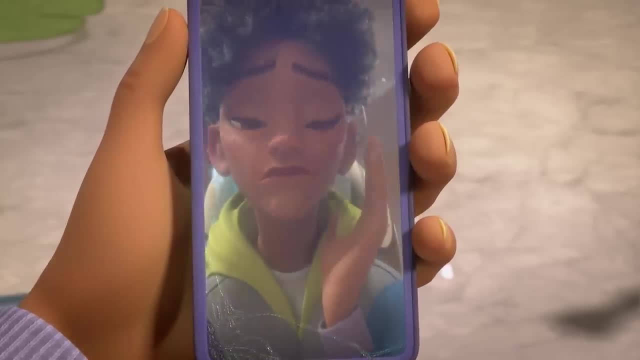 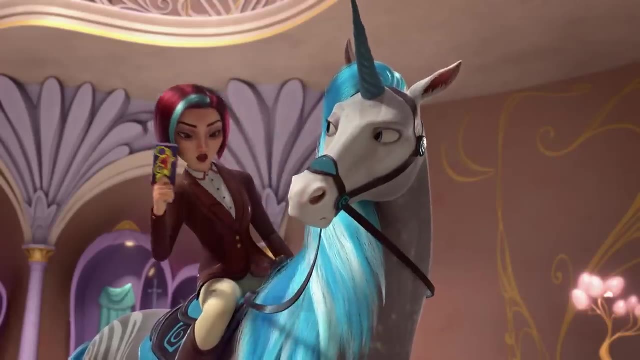 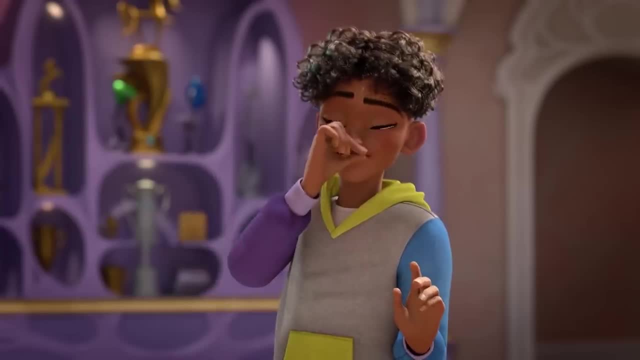 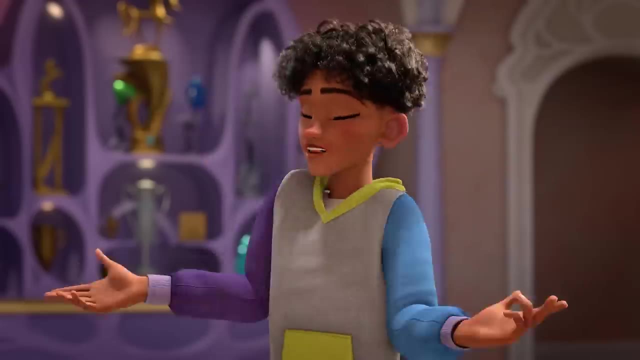 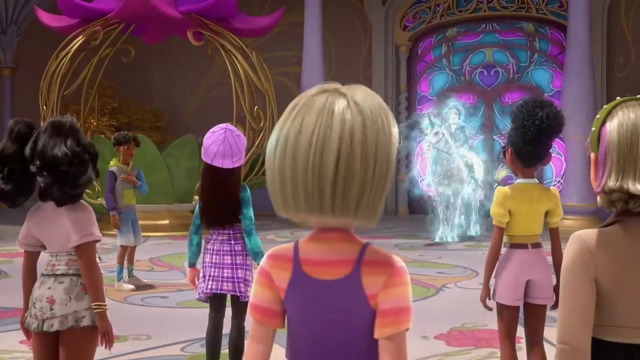 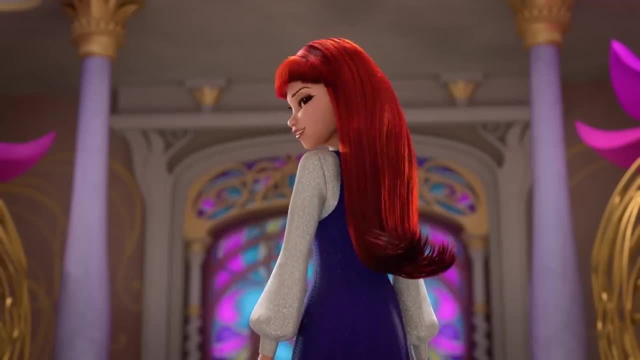 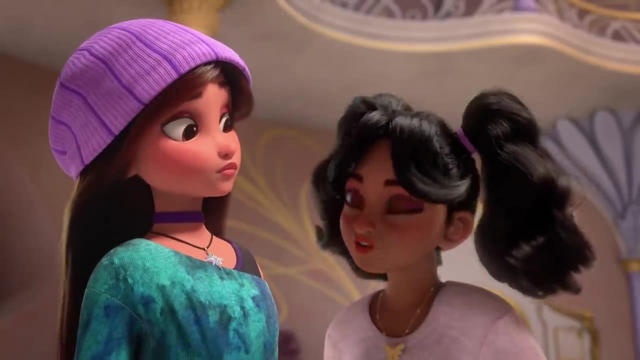 In case you didn't notice, there are like people here. Who is she? That's Valentina. She's not Valentina, She's like a super legacy. Her relatives were some of the founders of Unicorn Academy. Her aunt is Ms Fury, the magic teacher. 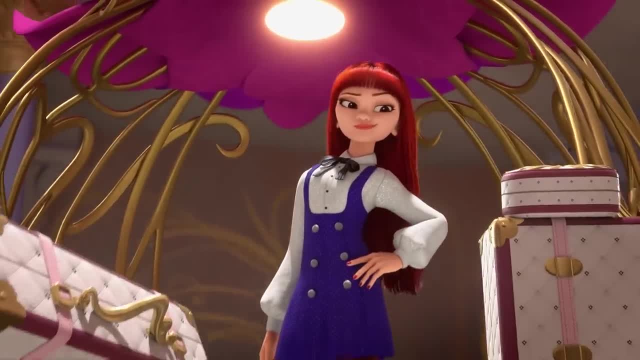 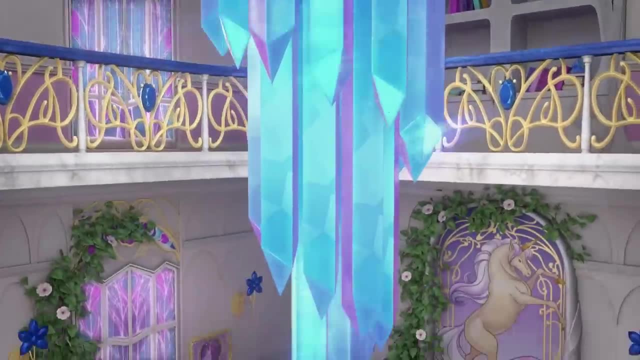 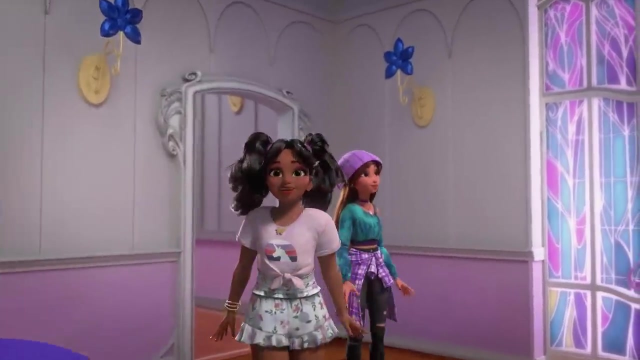 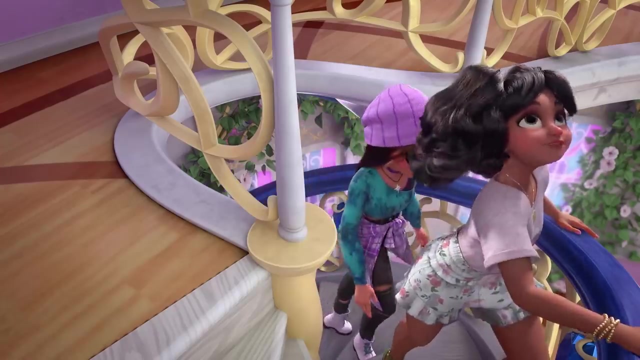 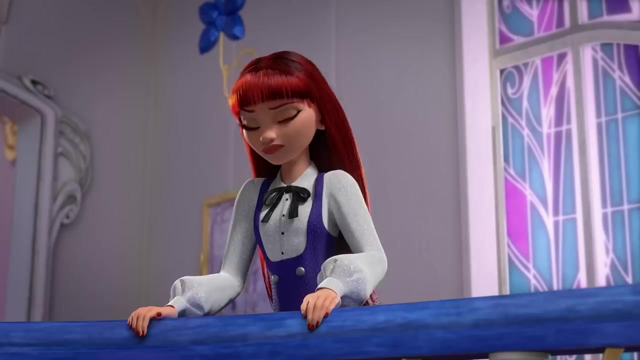 Valentina is basically Unicorn Academy royalty and definitely not used to getting called out Whoa, Whoa. I could live here, Nice. I hope my room's near the fridge. The energy in this room is amazing. How's the energy now? 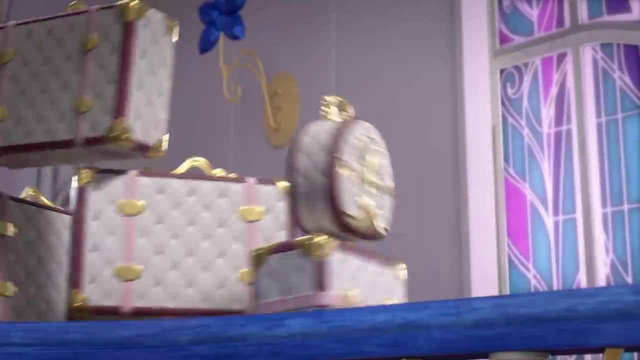 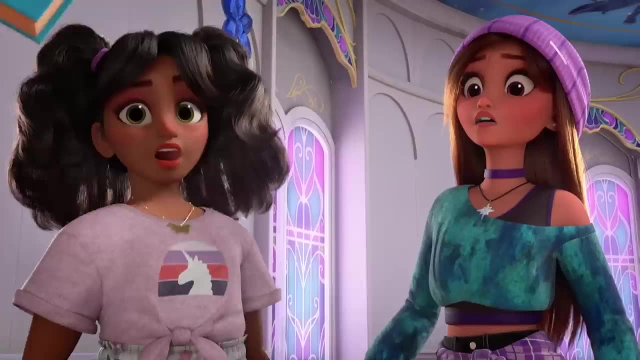 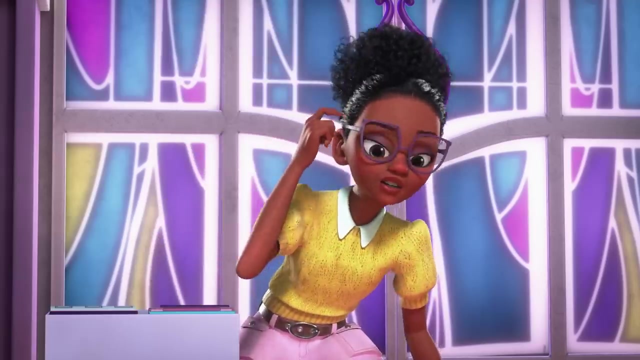 Great, This'll be fun. I need a library. stat Whoa. I knew something was up. when I got an invitation for a riding academy- and I've never been on a horse in my life- I had a hunch this was some sort of elite. 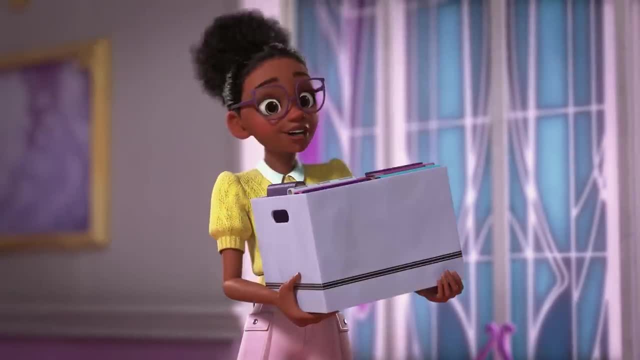 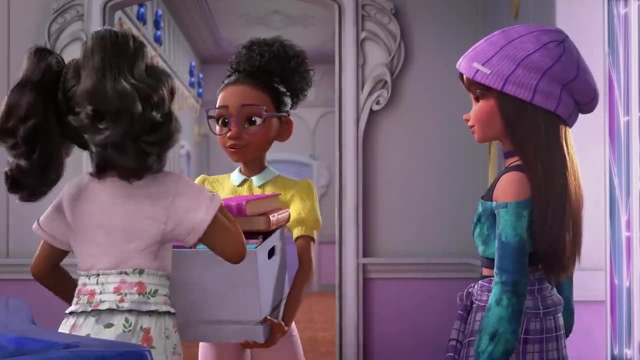 secret school. I was thinking a scientific government thing, code breaking, rocket building. but unicorns and magic mind blown. Phew, Glad I'm not the only one. I'm Ava. This is Sophia. I'm Layla. Okay, I better get unpacking, organizing. 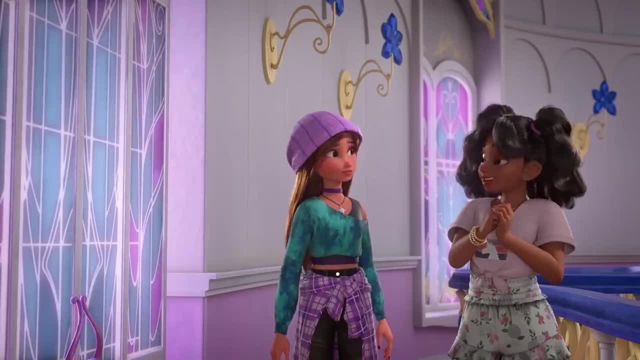 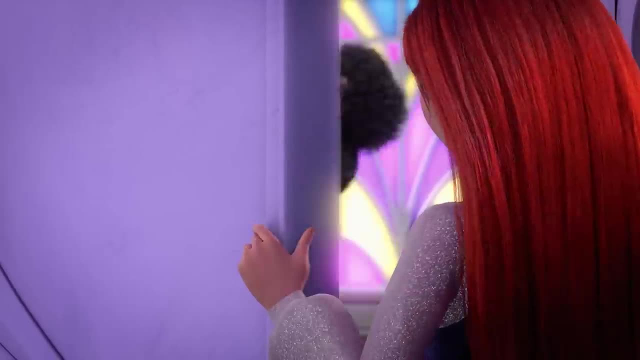 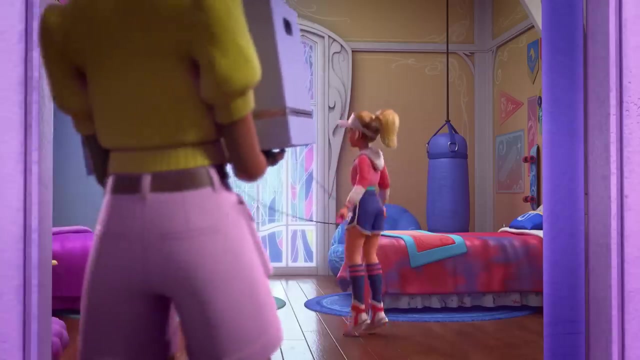 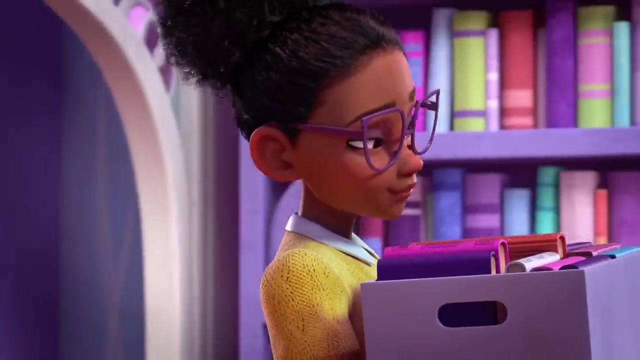 and well, let's be honest, reorganizing. Oh hi, Are we roommates? I don't do roommates. Hey, is this my room? No, Yes, Oh, so many books. What's up, dude? 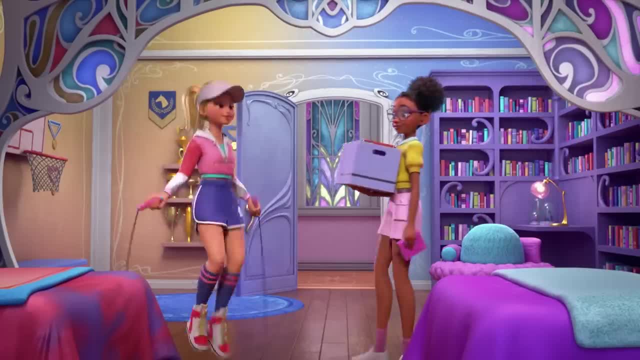 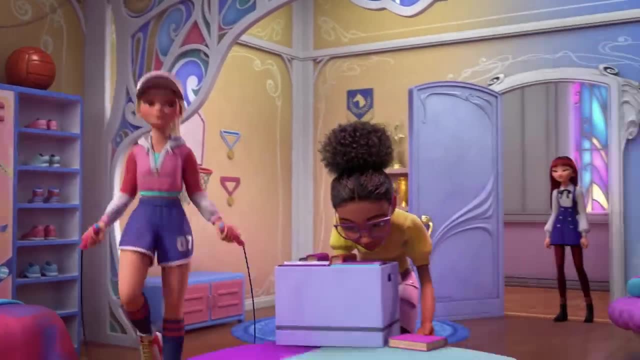 I'm Isabelle. That's impressive. Barely a warm up. What about you, roomie? You work out? Does speed reading count? Just curious, is this an all the time thing? Woo, nope, Just a couple hours at 5 am. 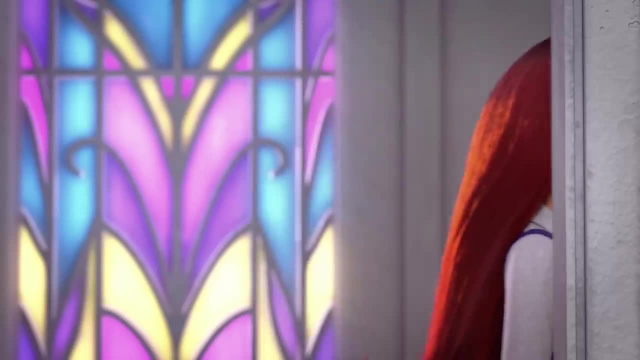 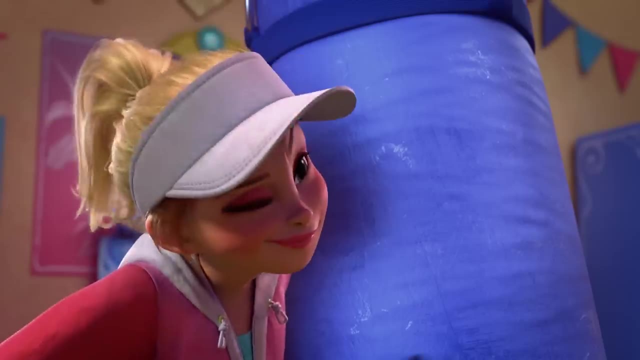 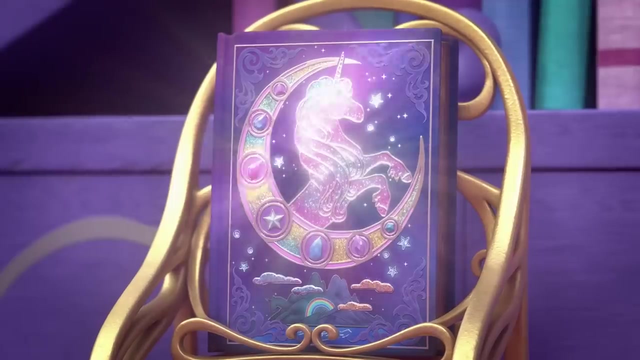 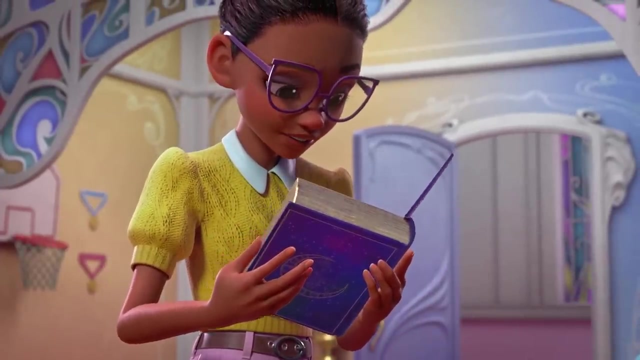 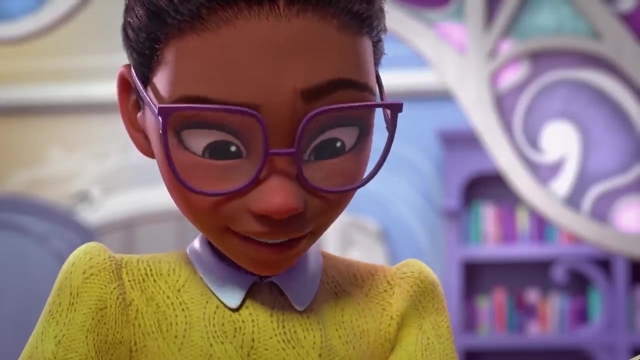 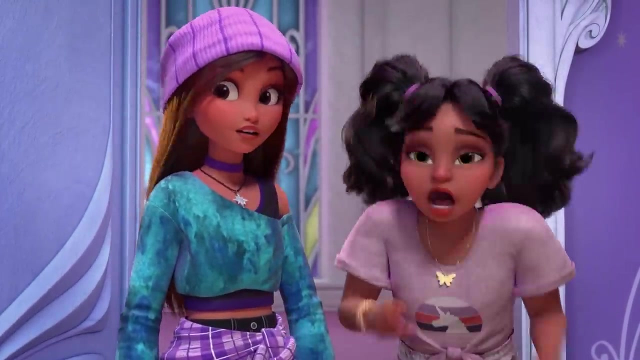 But not every day, Ah great. On the other days I do K-boxing. Sparkle book- a comprehensive guide to Unicorn Island. Can someone fall in love with a book? Because I'm in love with a book. They decorate our rooms to match our personalities and whoa. 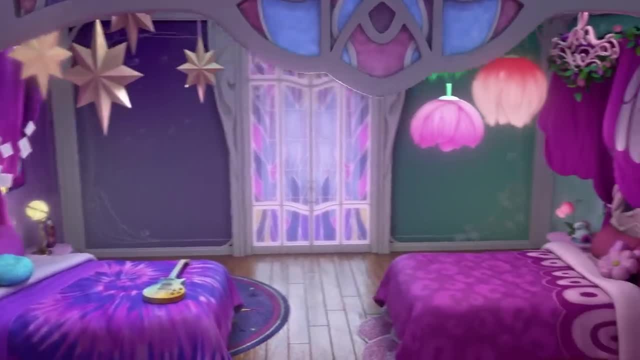 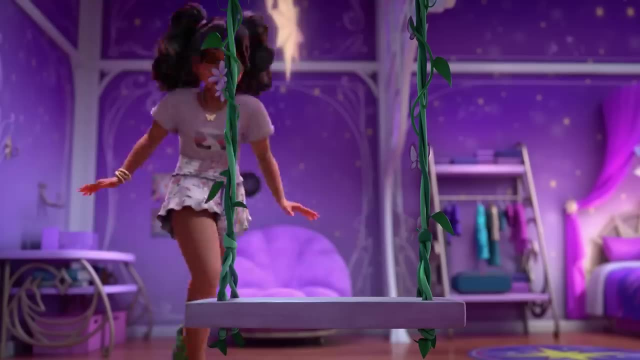 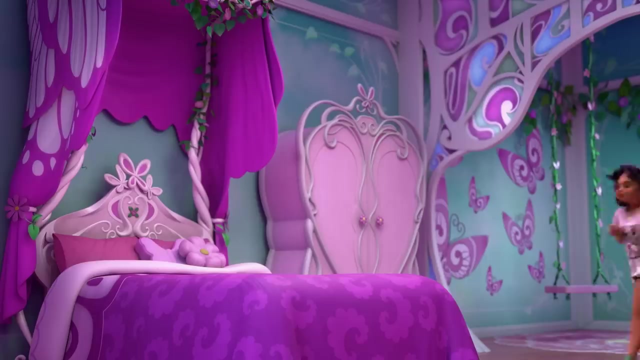 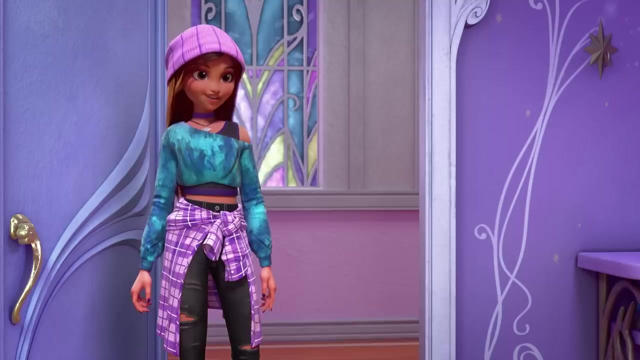 This place is so so- wow, I love, love, love it. Wow. This is so so so- wow, I love, love, love it. Wow. Oh, look at this Amazing Whoa Flowers. 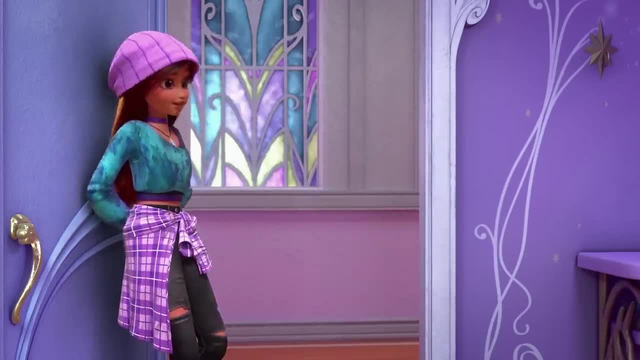 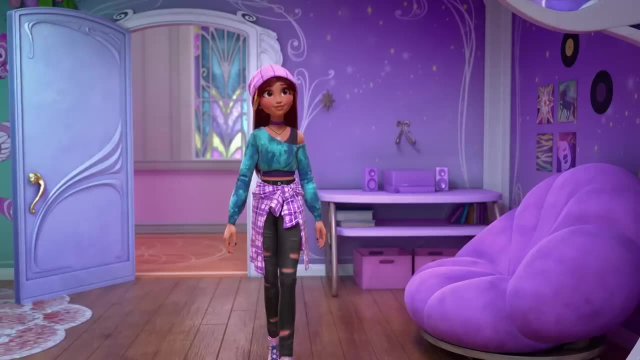 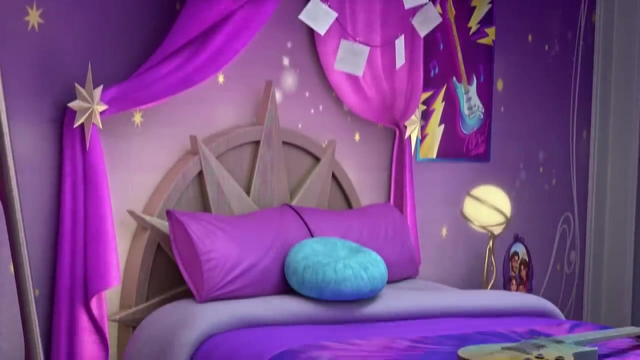 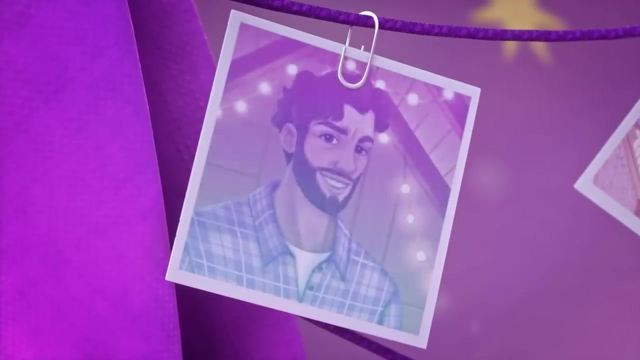 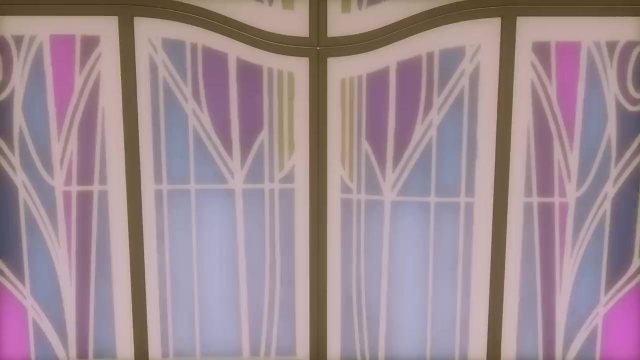 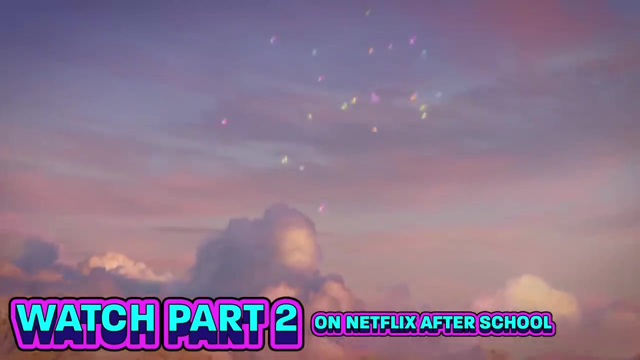 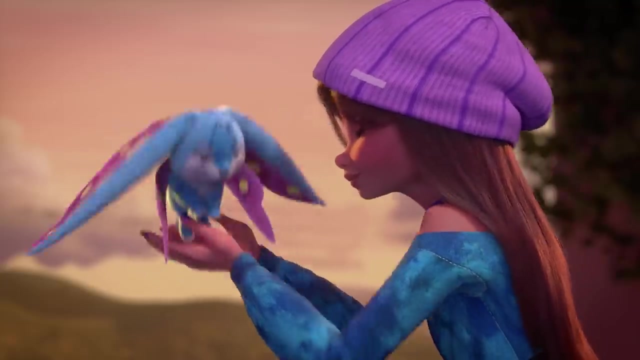 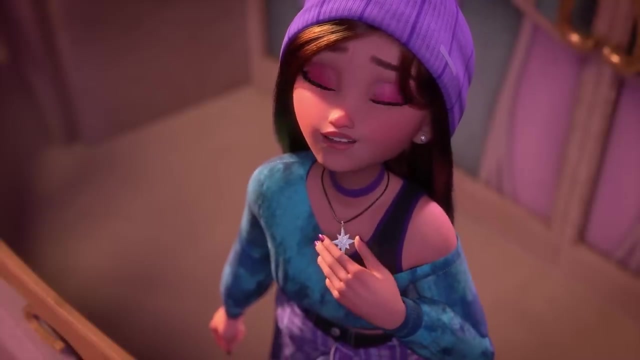 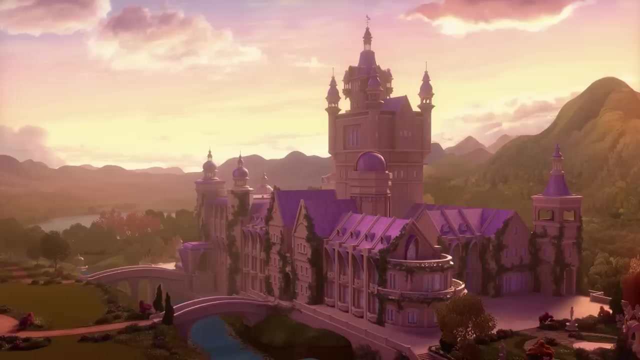 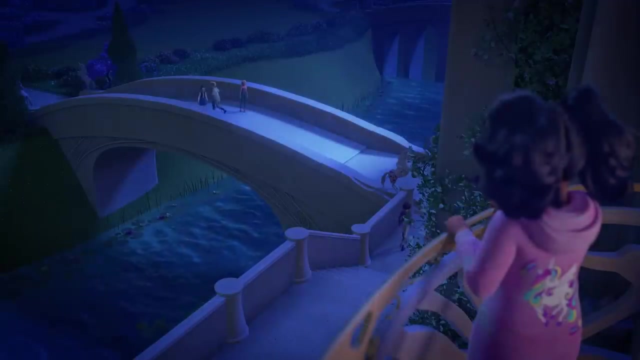 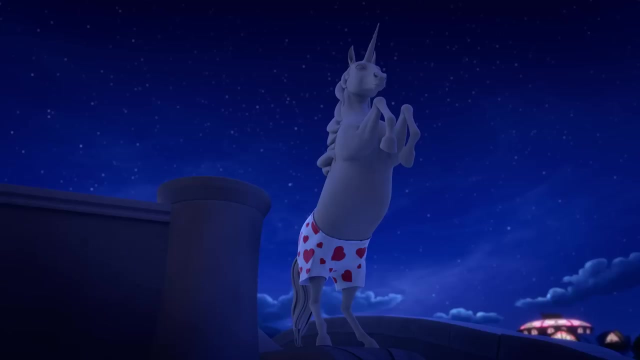 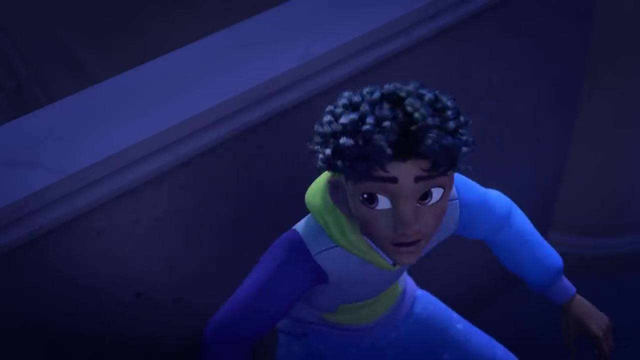 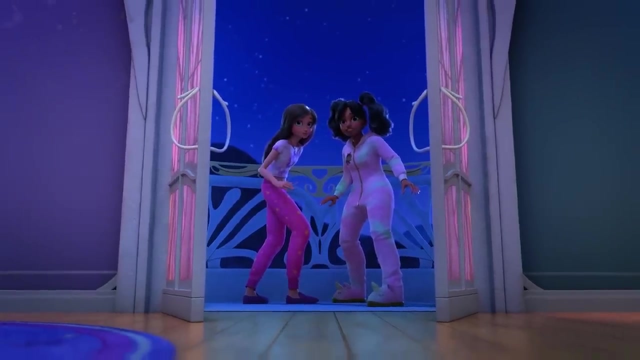 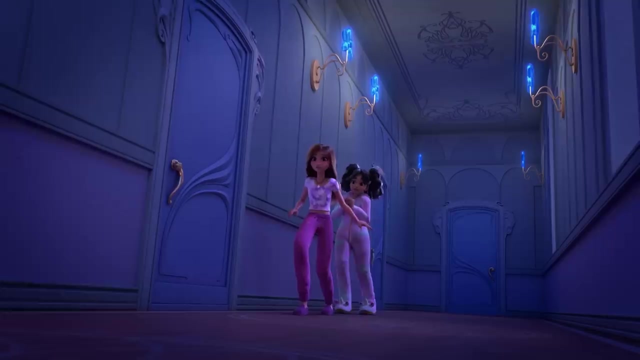 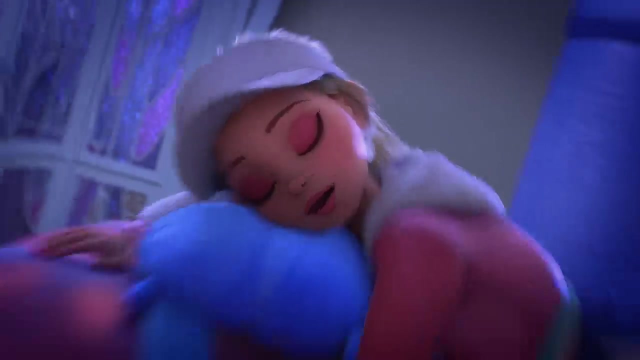 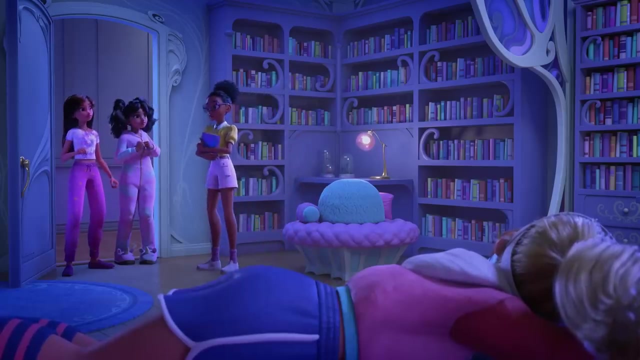 Yeah, no, Definitely not my room. Huh, It's perfect, Perfect. Wow, Dad, I think I found my extraordinary. Whichever student is responsible for this will face consequences. Hahaha, What was that? Sorry, Since we're training to be Unicorn Island heroes. I'm just reading about some of the villains. 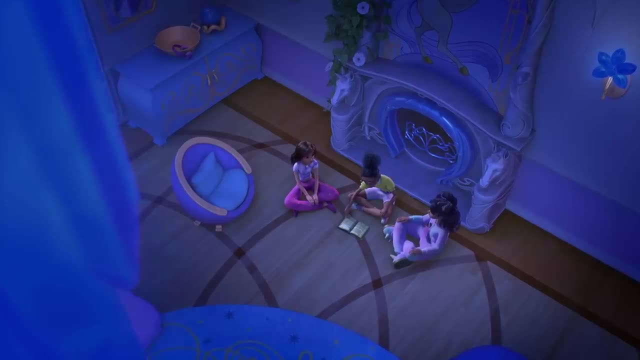 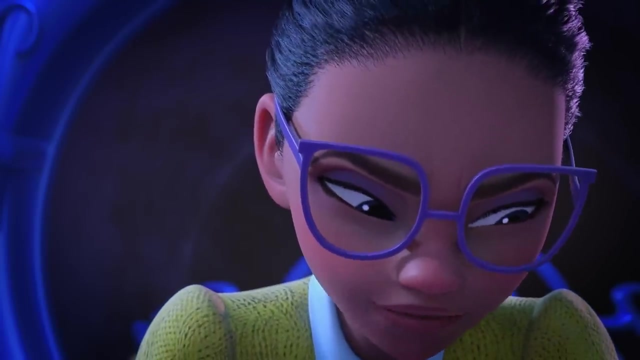 So this place isn't all lollipops and rainbows. Um no, There are frost goblins, swamp shifters, something called a silver mountain cyclops Big list here. They come from the island kingdom of Grimoria. 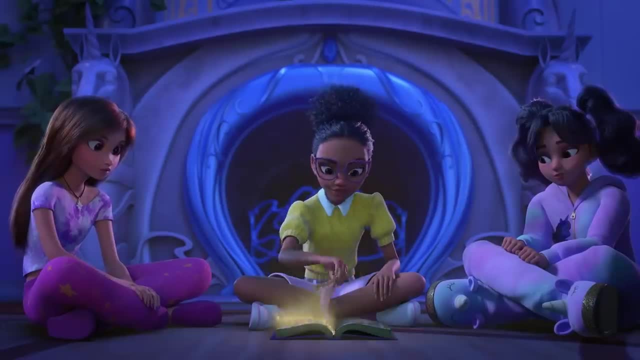 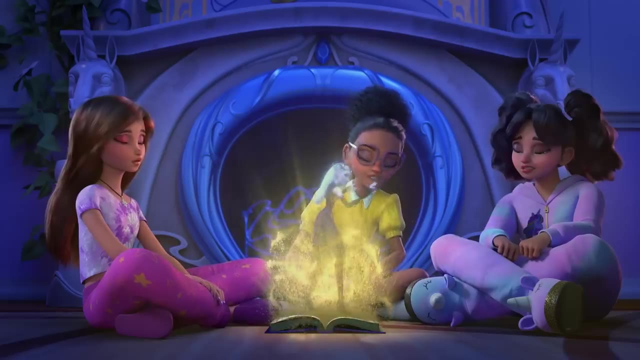 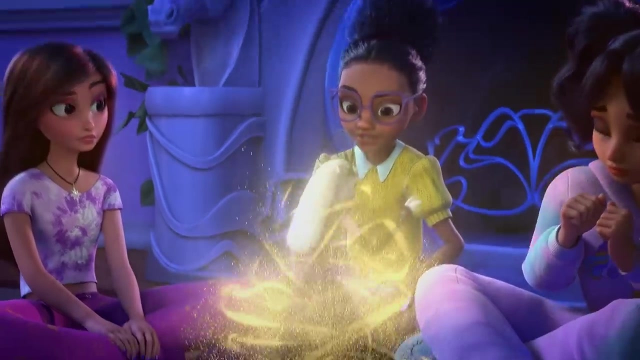 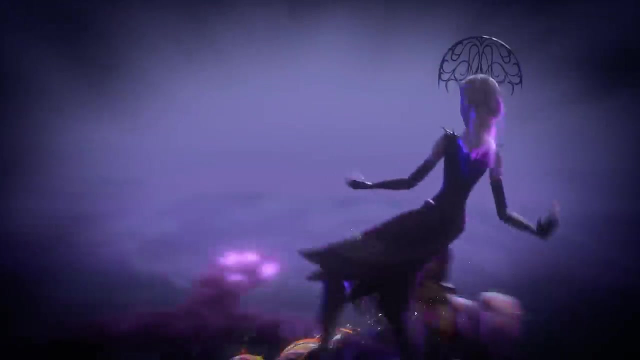 Grimoria, Home base of something called Grim Magic. Who is that? Raven Zella, Queen of Grimoria. Uh, I know it's not real, but she's giving me the creeps. She almost took over Unicorn Island, But a brave unicorn rider defeated her and locked her away in the Cell of Eternity. 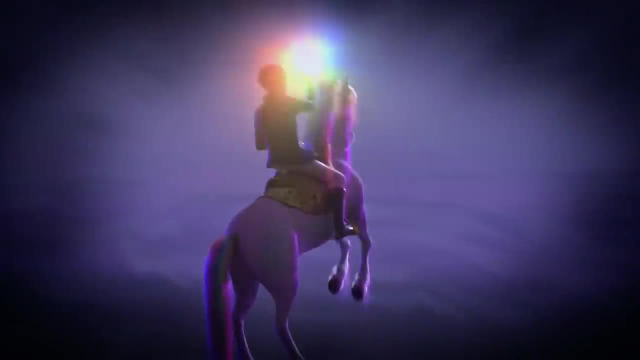 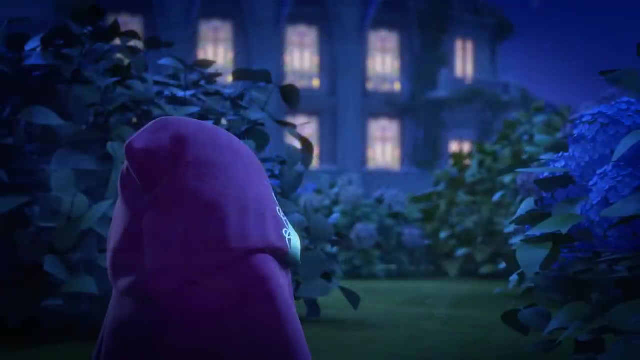 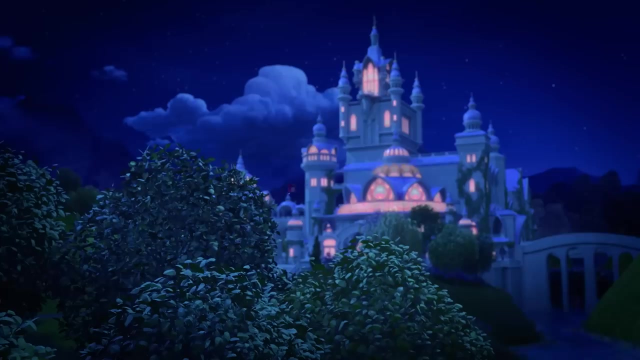 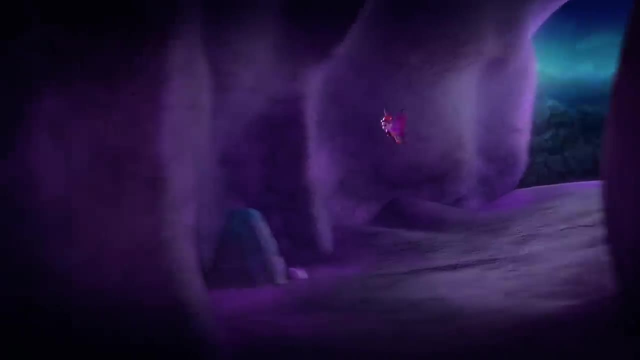 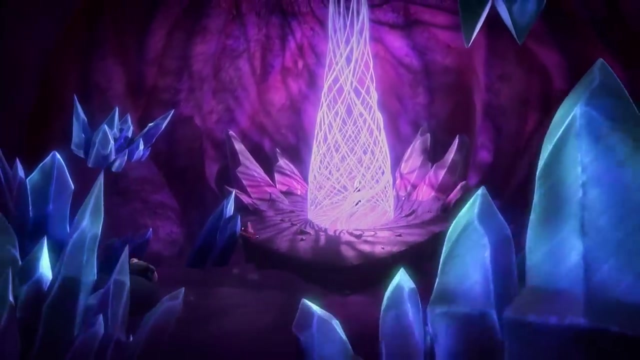 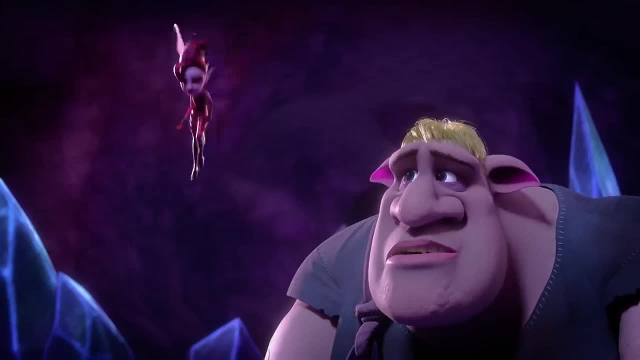 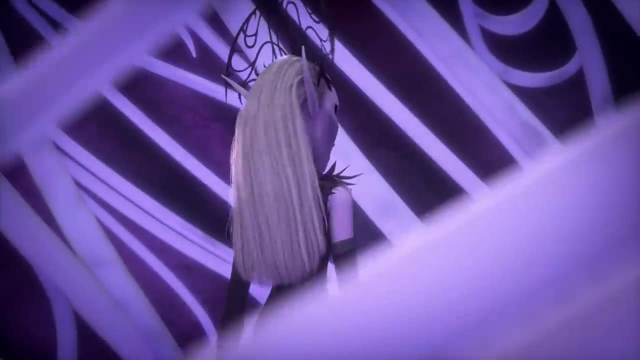 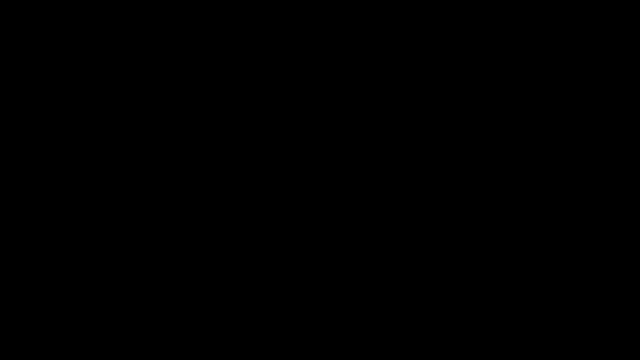 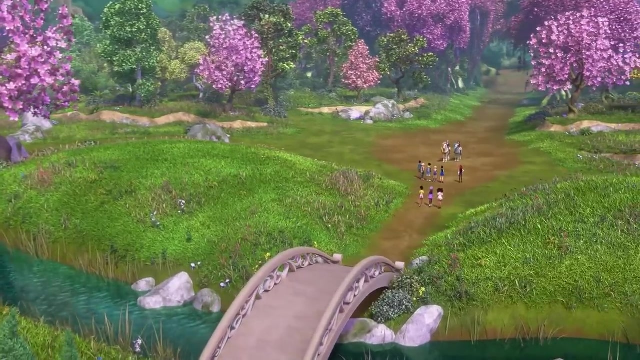 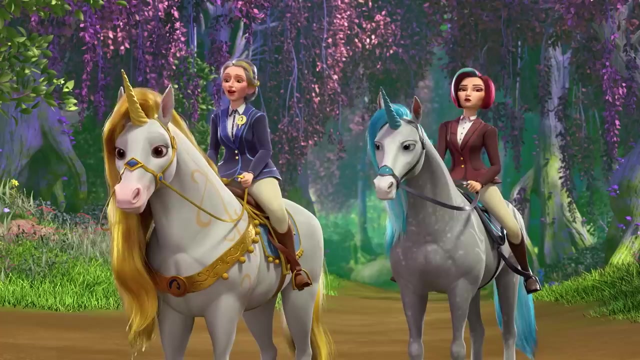 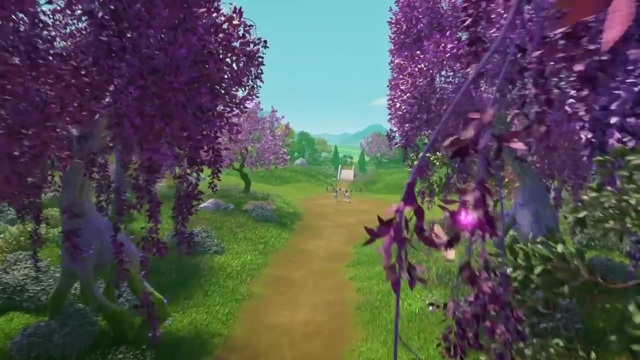 Oh, I have a message for our Queen. It's time. Well, well, How lovely. good morning, students, and welcome to wonderwood forest, where the unicorns of this island roam, and today you will discover if one of those unicorns is destined to be yours. 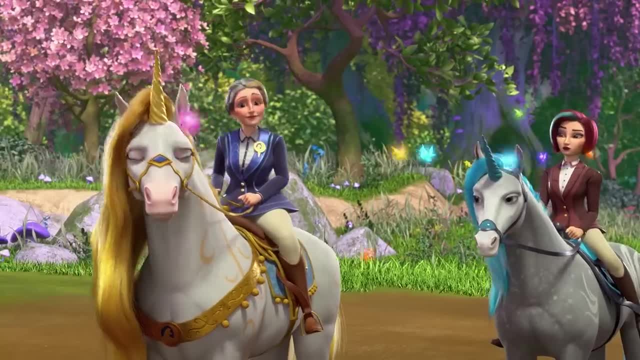 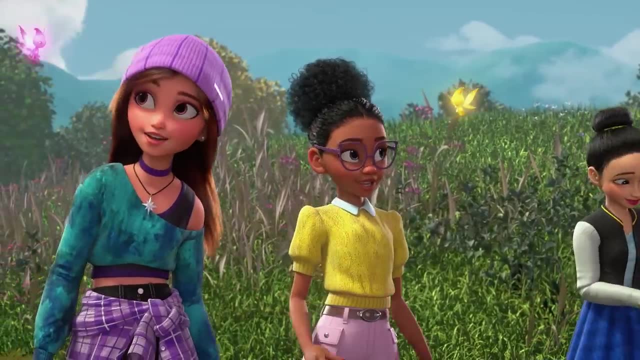 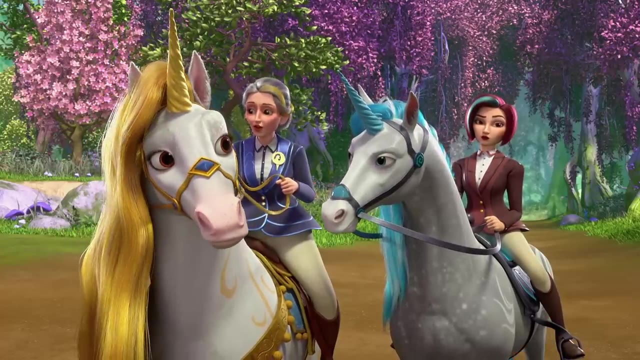 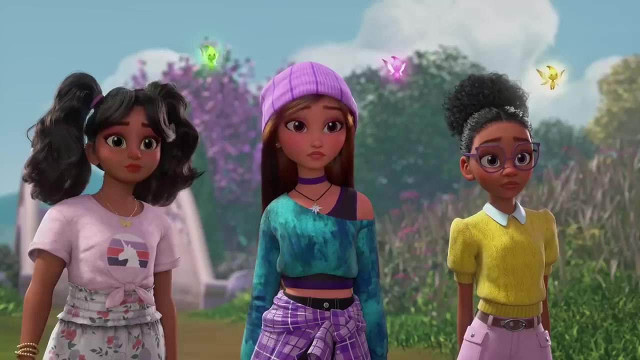 aha right on time. if you find the unicorn that is your destined match, the fake fairy will glow brighter. for those of you who match with a unicorn, you'll get your uniforms at the enchanted archway this afternoon. for those who don't, becoming a unicorn rider was not your destiny and you will. 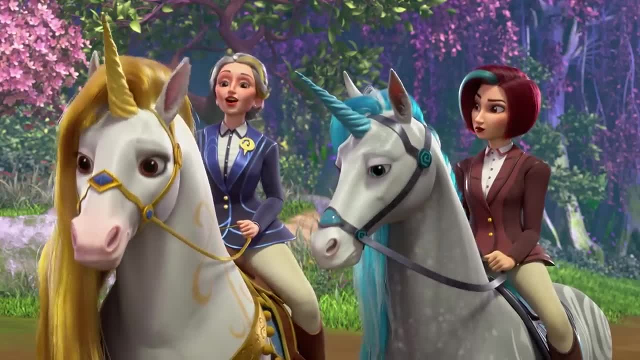 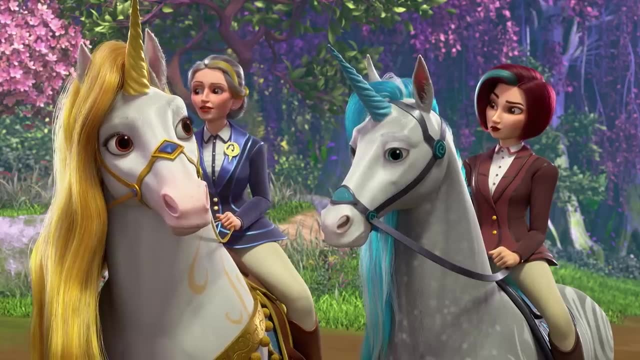 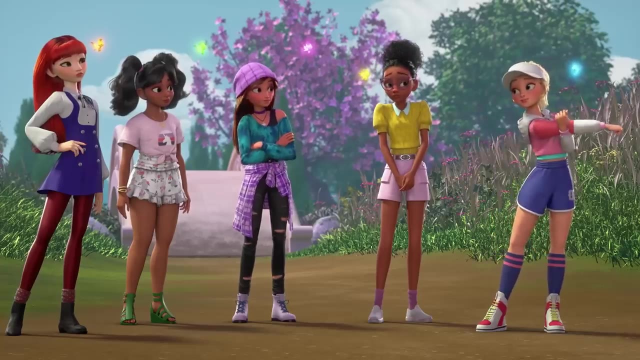 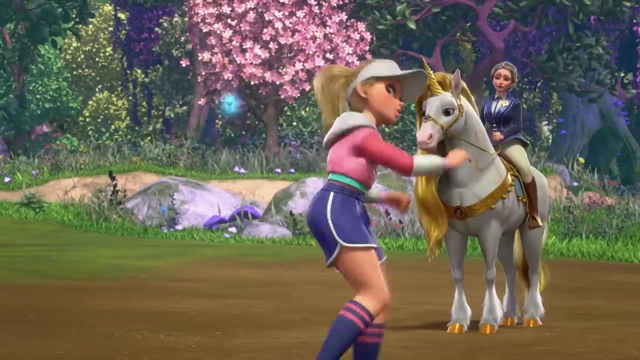 be sent home. don't worry, just follow me. follow your heart and see if it leads you to a unicorn. but remember, as you search for your unicorn, you must not go beyond the shimmerstone wall. last one to find a unicorn buys lunch. i mean, food here is free. but you're on, your destiny awaits good luck. come on, let's go. 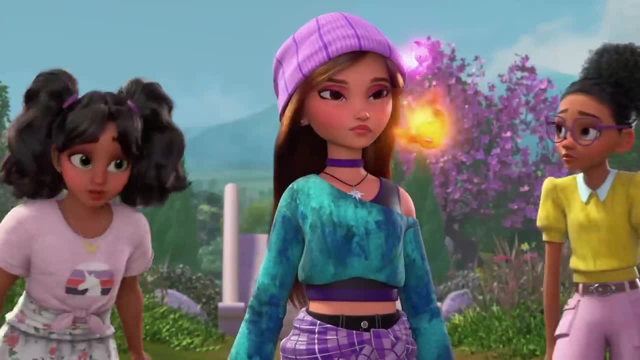 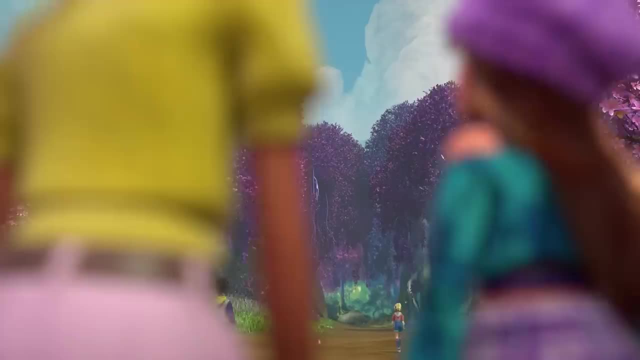 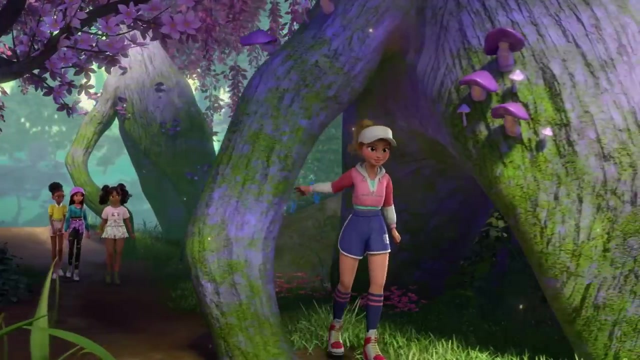 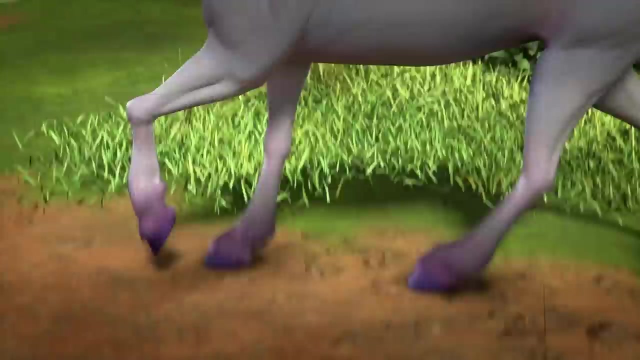 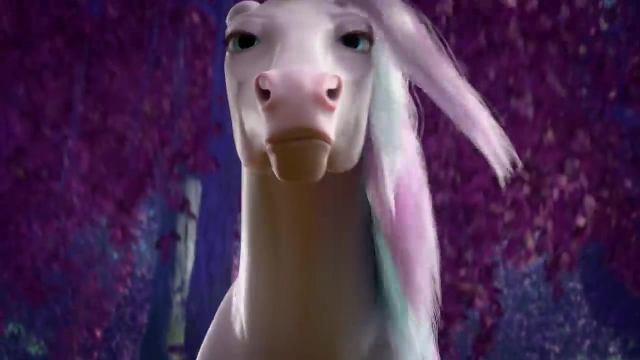 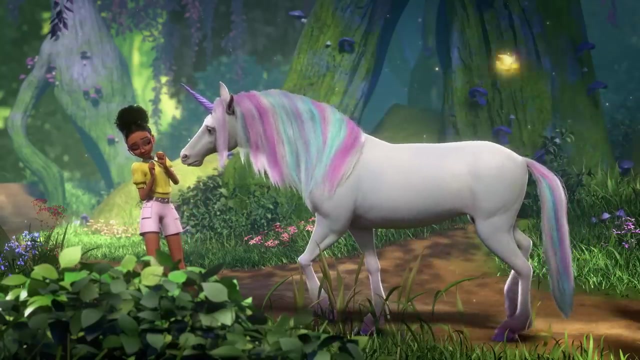 oh, i can't wait to meet the unicorns we match with. if we match- yeah, no pressure or anything- we will find unicorns, we will find unicorns, we will find unicorns fast, strong, powerful. yup, i have found mine, my unicorn, so it looks like we're uh um team. 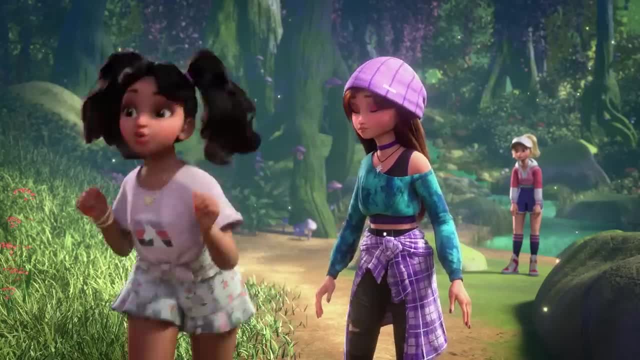 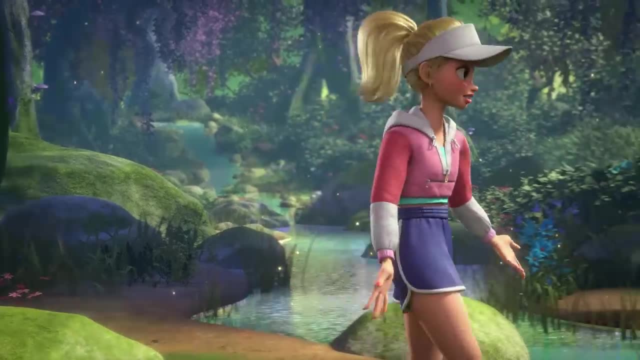 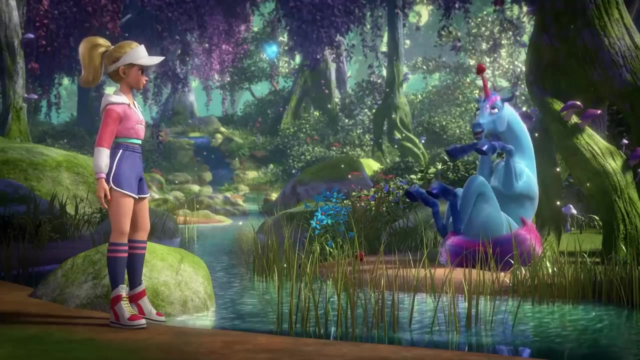 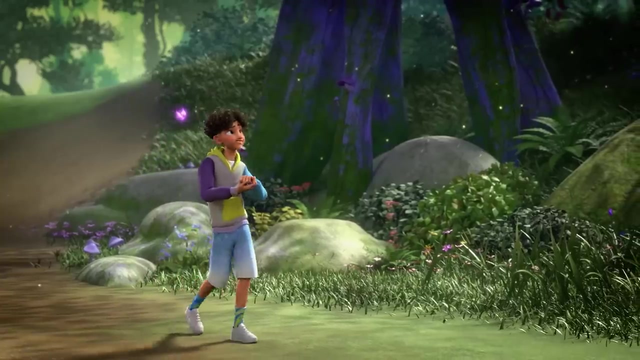 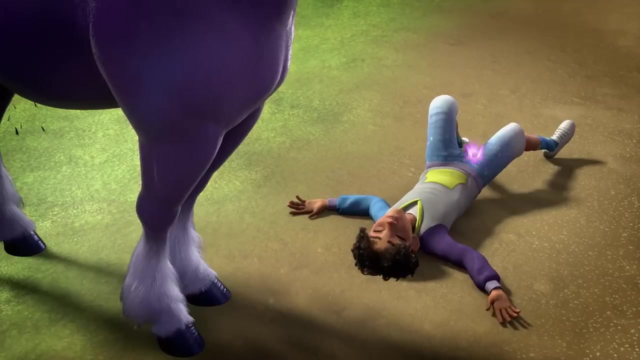 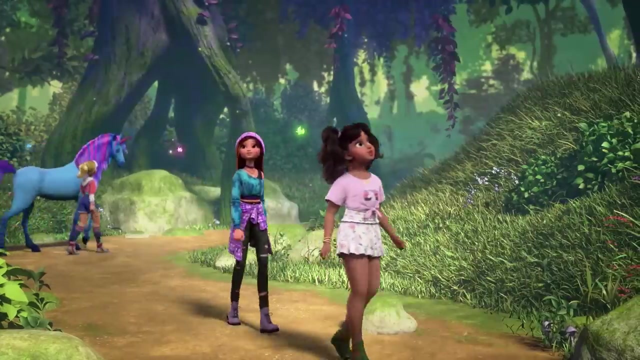 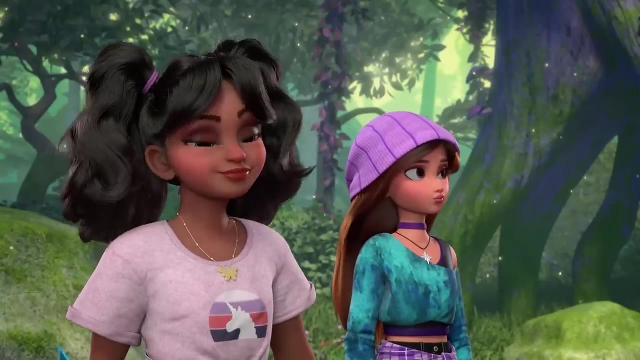 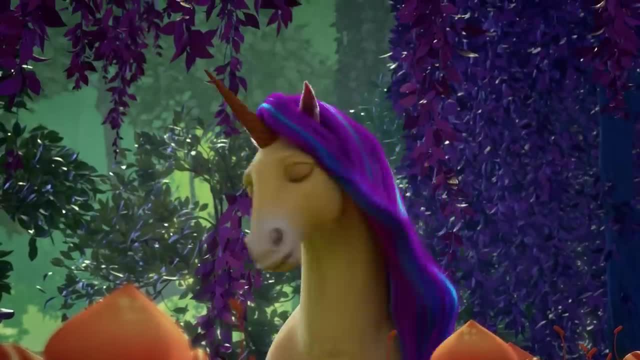 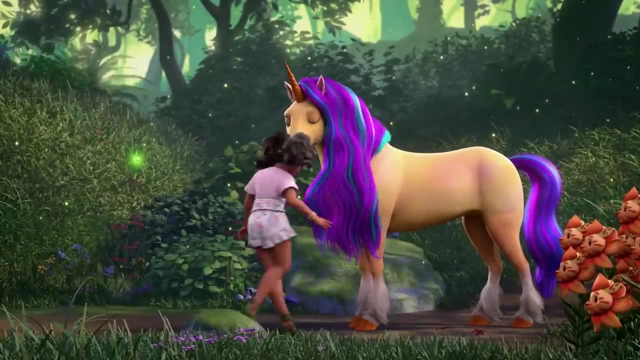 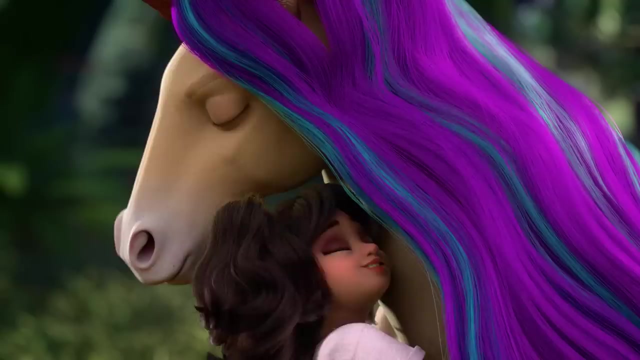 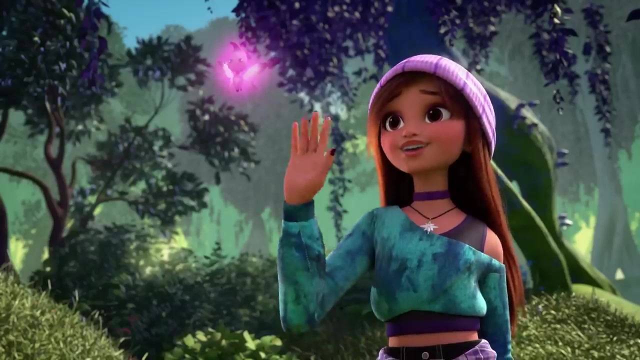 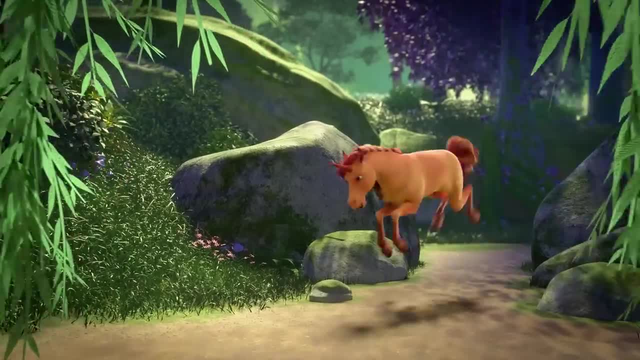 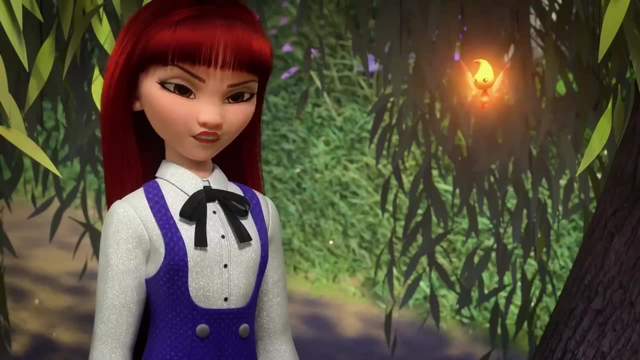 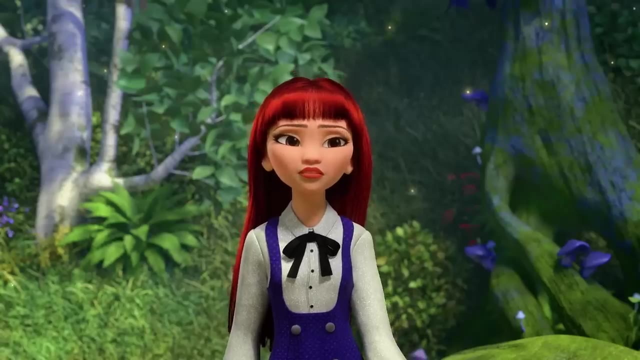 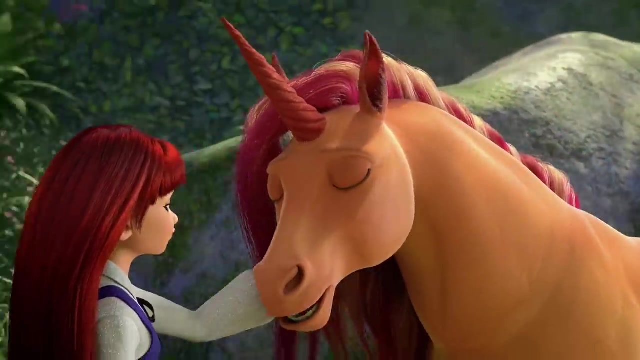 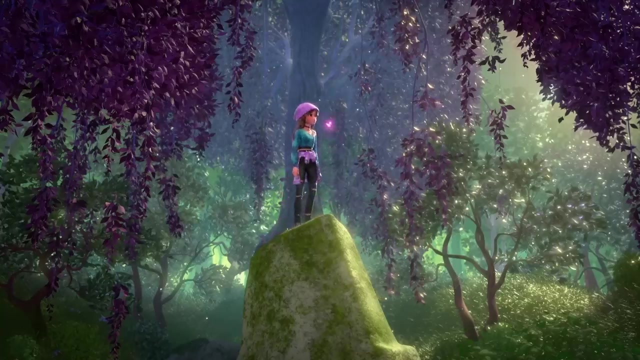 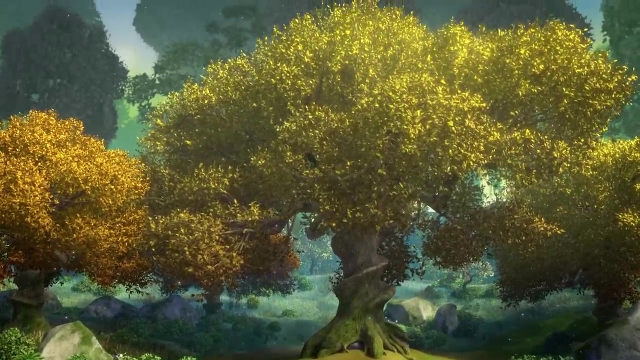 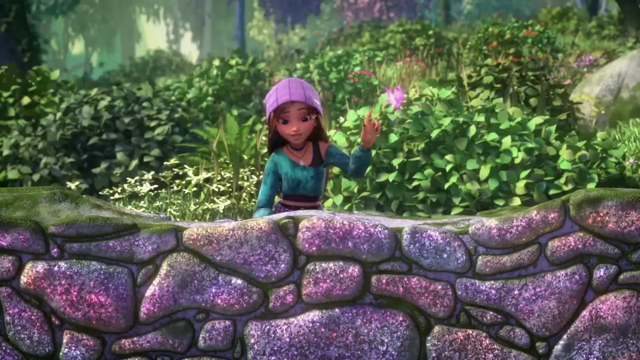 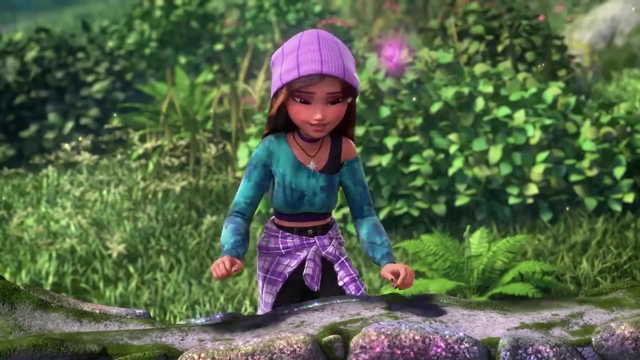 I want to get it out of the way. aah, Hmm, Fierce, I like it. Hmm, You can do this, Sophia, You just need a better view. I'm guessing this is the Shimmerstone Wall. Miss Primrose said not to cross it, but this is a unicorn-fighting emergency. 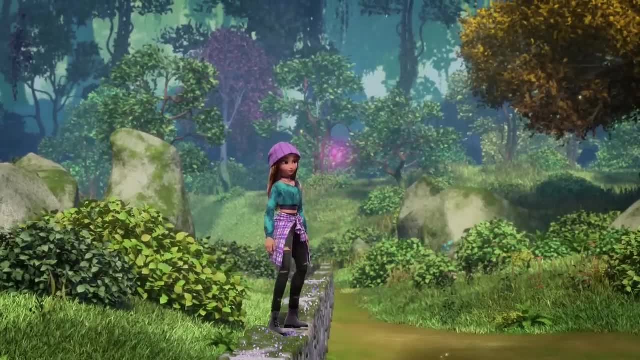 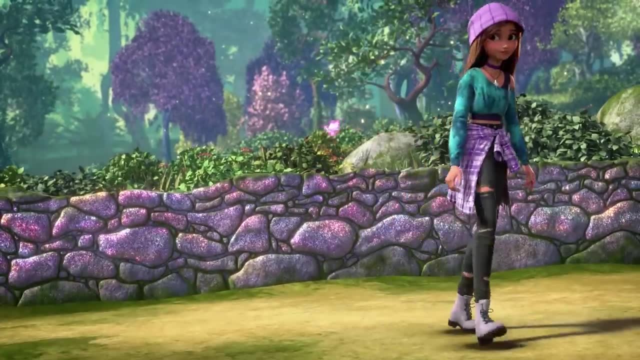 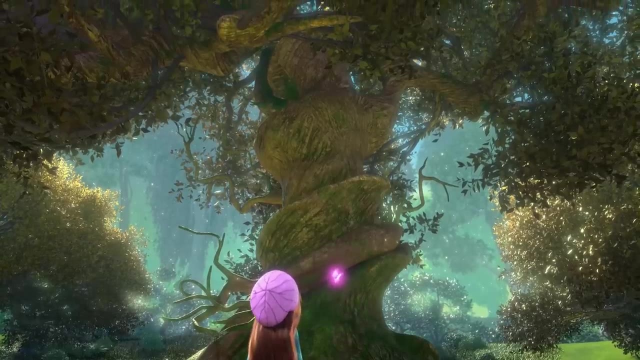 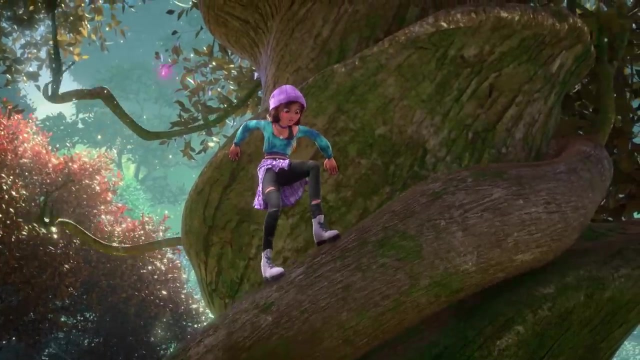 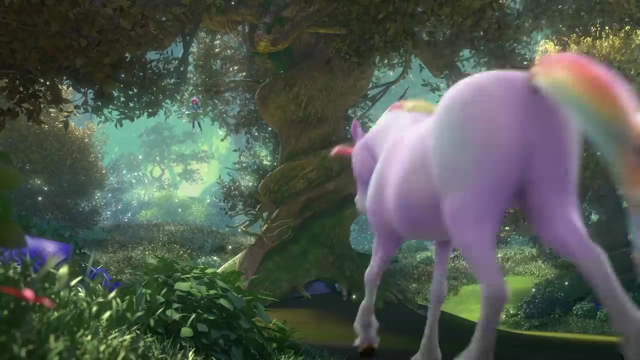 And if I'm going to be fighting evil, I think I can handle a quick trip out of bounds. Ha, I'm going to have to get out of here. Thanks, Ugh, So good. Huh, Huh, Aaah.